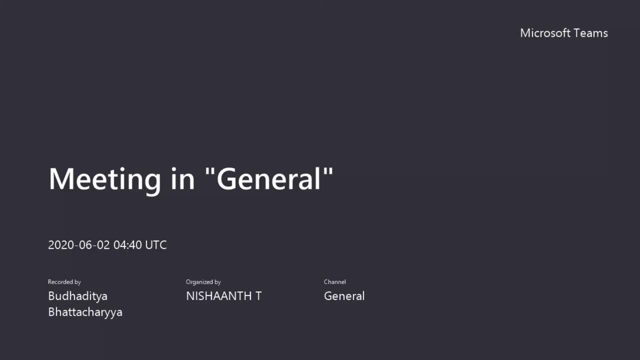 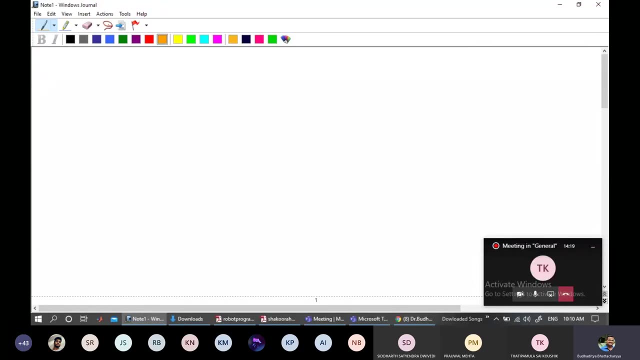 This white screen. to be honest, can anyone please confirm this? Yes, sir, Yes sir, Fine, fine. So till this point, what we had done is primarily the few modules. If you remember the first way, we started off with the basics. 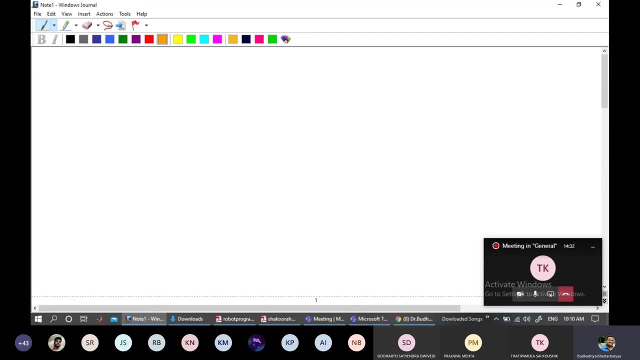 Then we went to the actuators part. Then we had a discussion on the sensors modules, different sensors using robotics. Then the primary discussion of CAT II portion was based on the DH parameters as well as the different types of the Denewitt-Hertenberg rules, the rules to find with different set. 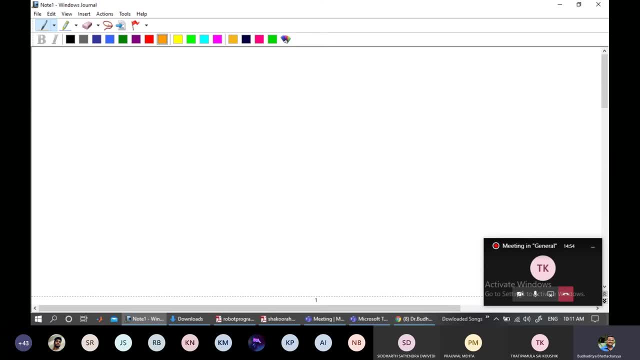 of planes: the inverse kinematics, the forward kinematics. So this was what we already did. So let us start with our discussion today with the fourth module, to be honest, and that is called as the path, Path planning. 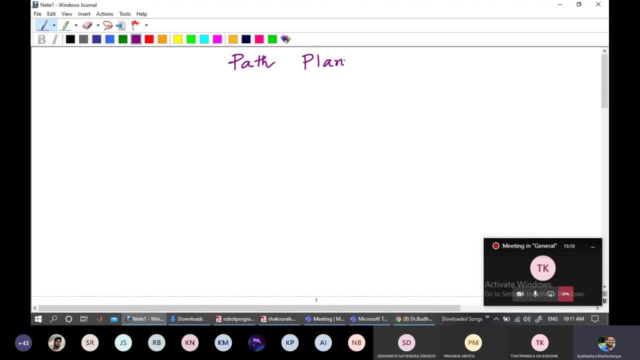 Okay, So this is the subject. Just see whether it is visible to you, I guess. so It should be visible. Yes, sir, Fine, fine, Because I have been taking classes based on this. only So everyone got it through. 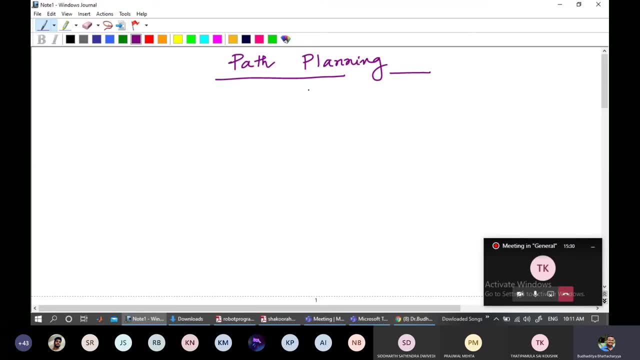 So what is path planning? So path planning: in the previous module we have mostly focused on how to do the path planning, But how? we have mostly focused on how the end effector. the end effector would drop something or pick up something, maybe, or drop or pick up something to a given point. 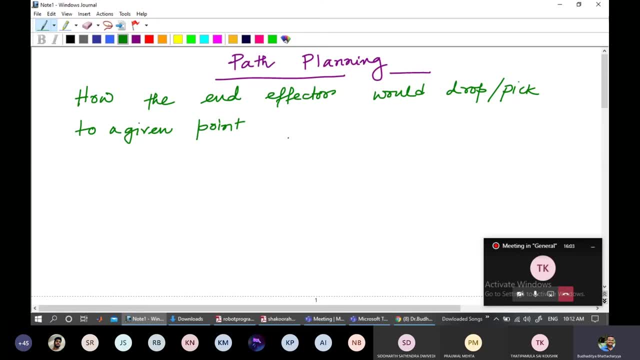 So just to recap on what we have done in forward and reverse kinematics for that matter, how the end effector would drop, Okay, How the end effector would drop or pick up a particular object, maybe to a given point, based on the given location. 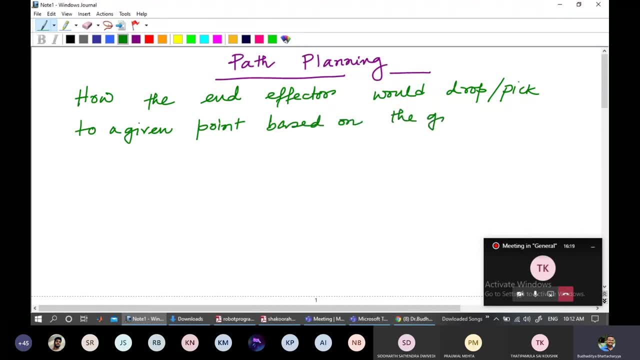 So based on the given location, Okay. Oh, another thing, just for my own confirmation. I will be asking few questions in between, Okay, So that also. I will make a note of the person answering it so that I can keep it as a bonus. 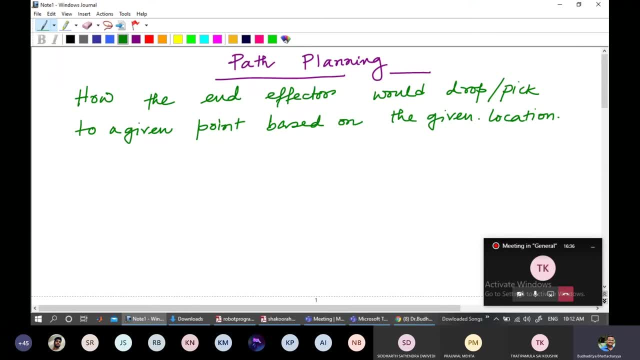 marks for adding up to some extent After the end of all our classes, so that I can add this marks extra marks for the answers in your CAT 1 or CAT 2 or for your anywhere where your marks is lagging, I will. 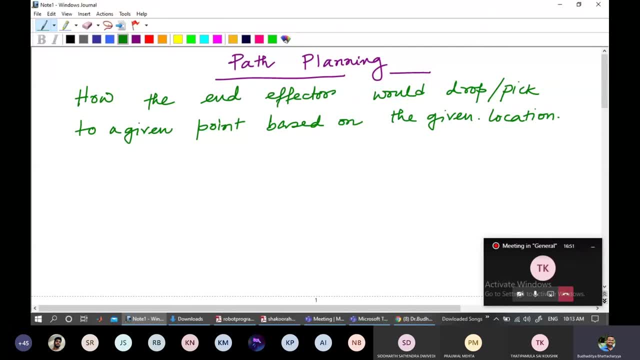 add those additional marks there as well. So I will be asking you. So just keep in mind on what I am talking about. I will be asking randomly to any one of you or in general. So this is what we had done so far. 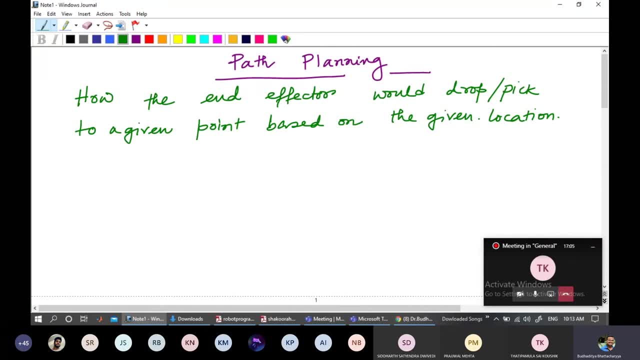 Okay, Okay, The end effector would pick up or drop something at a given Point based on the location. Now, the path planning, or this particular module, deals with that which. the path, Okay, Please note it down. The path through which, through which the end effector 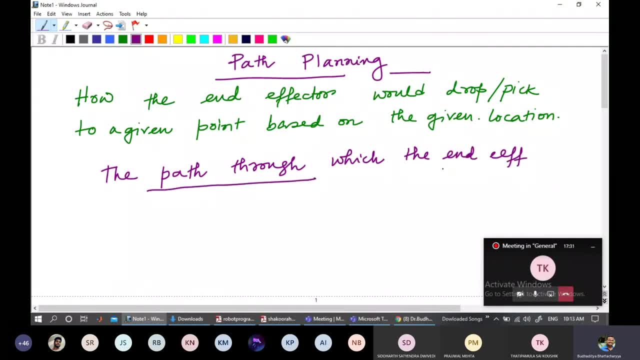 Okay. So this is what the highlighting point is: The path through which the end effector is moving, Okay, Or positioning itself, because we only knew that it will pick or it will drop something, but what is the path through which it will pass in order to do that? is what is important. 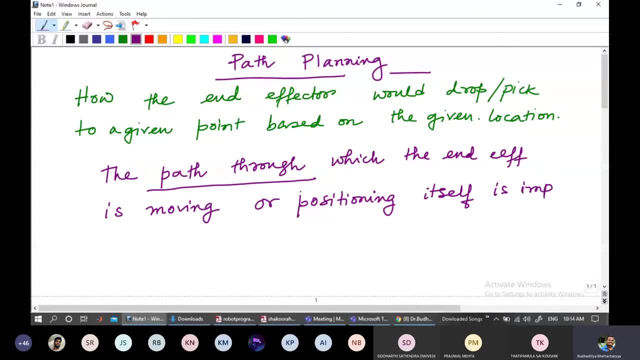 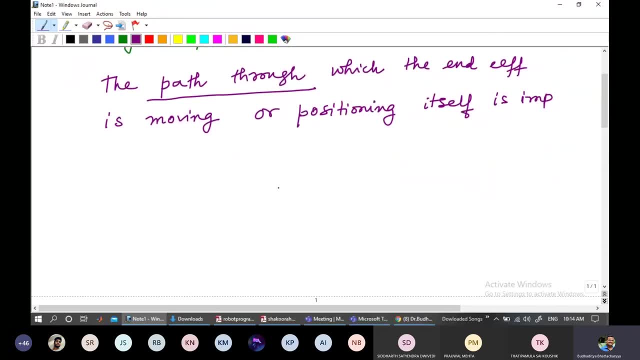 Is important And that is where, and that is where we are talking about the path planning nature. So I guess you, you, you are now kind of understood that. What is the role? What is the role of this path planning in our scenario? 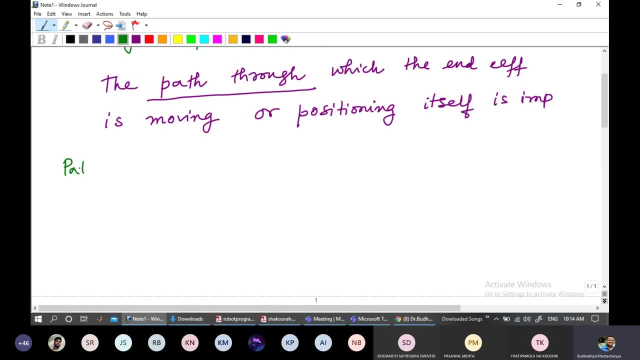 So let me just give you the formal definition of path planning then. So path planning as a definition is: it is a process, process to figure out. process to figure out the point in space, The points in space, Okay, Points in space. 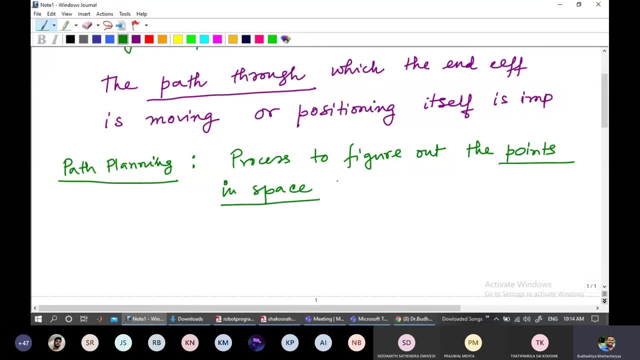 This is important- through which? through which the end effectors, the end effectors- will pass Okay, So, so this is, this is what the path planning is Okay, but there is another thing to it, and that is called as another set of different mode of. 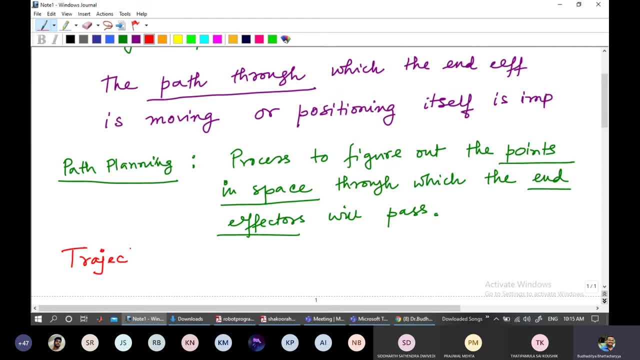 planning and that is called as trajectory planning. So we are now familiar with the path that the robot will follow, or the process that robot will follow in order to do some action. The trajectory planning is that when we add the velocity at which maybe an arm of a robot will, 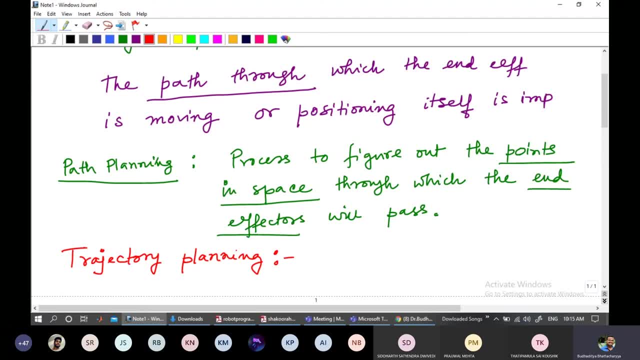 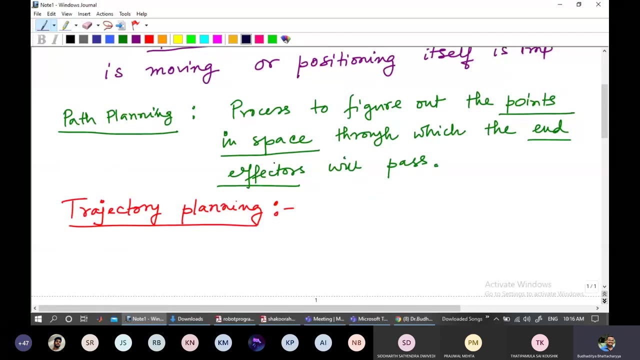 move, or maybe what will be the acceleration at the end? effective point Understood. So this is the difference. So the difference. this is a very common question that usually used to come in your robotics tournament as well- that what is the difference between these two? So 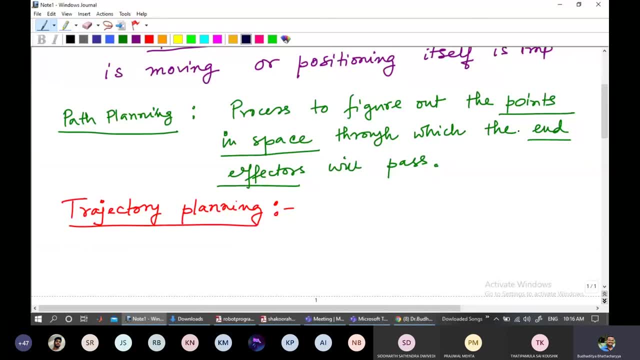 just to understand this: path planning is the process to figure out the points in space, whereas in trajectory planning it is the figuring out the velocity component of the end effector, motion along the path. So, ideally, what we can say that it is concerned about when each part or path must be attained. 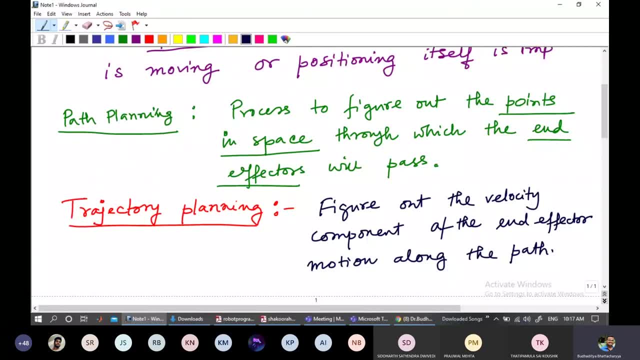 So, based on some timing, we will find out that what are the points that it has gone through? and we have to find out, we have to categorize that- what is the velocity at that particular point? So suppose I have a scenario like this. I will just give you a small example. 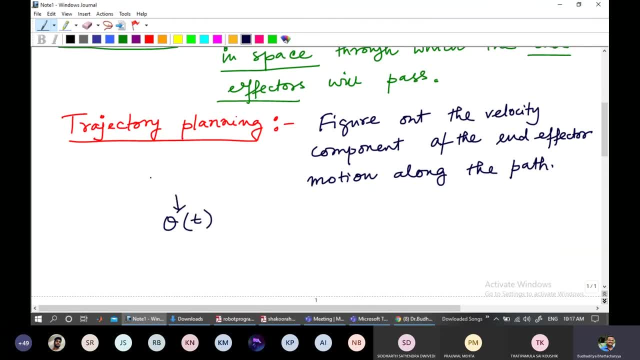 Suppose this is my theta t. Theta t is the velocity at which the robot is moving. So suppose the joint variable, if you remember the joint variable we used to calculate. So this is the amount of rotation that the rotary joint will have at a particular time, instance t. 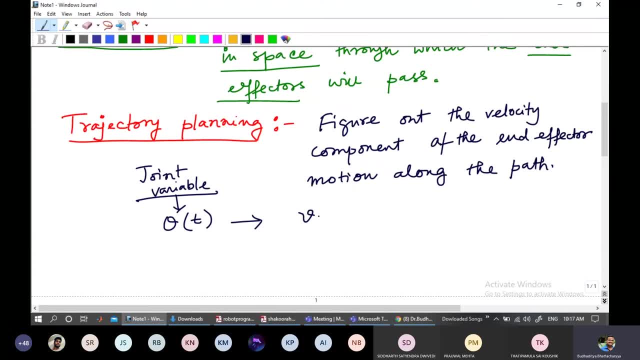 Now, at this point of time, suppose it has a velocity v1.. So we will also figure out that if this is theta 1, so what will be the theta 2, or the joint variable when, or maybe it is t1 at t2? 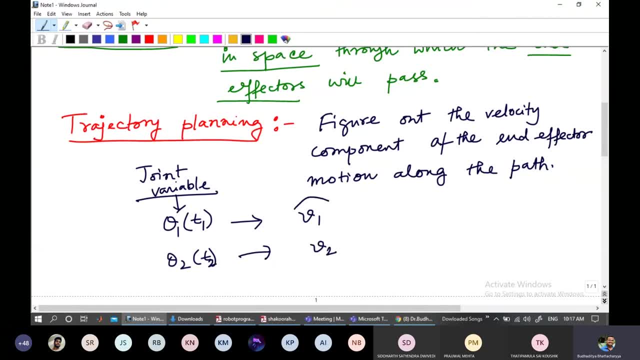 when the velocity becomes v2.. If you take these parameters into consideration and you try to plan, what is the path that it will traverse, that is, the physical parameters like velocity and acceleration. to be honest, these are the two parameters that usually is considered. we will consider that as a trajectory. 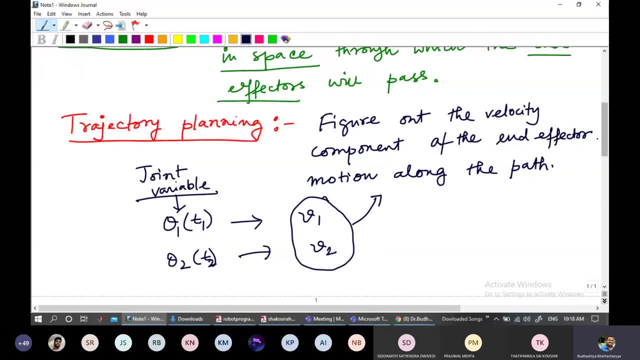 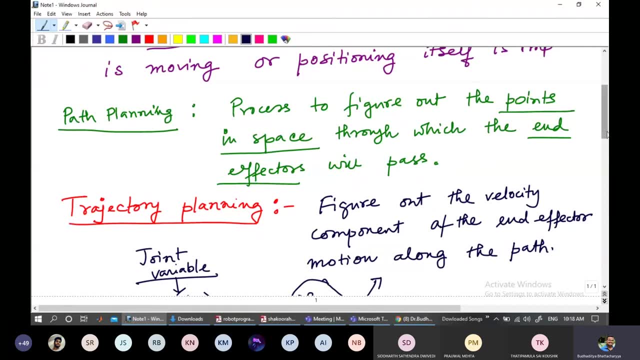 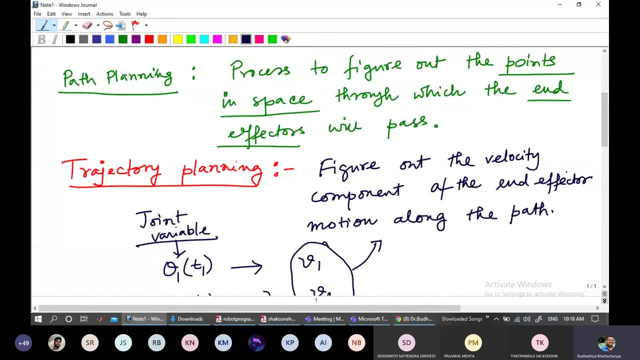 generation or trajectory planning clear. So this, till this point, what we have discussed is that the path planning is a path planning is basically a scenario where the robot- how, what is the path it will traverse and how it will traverse based on the physical parameters- is given by the trajectory planning. 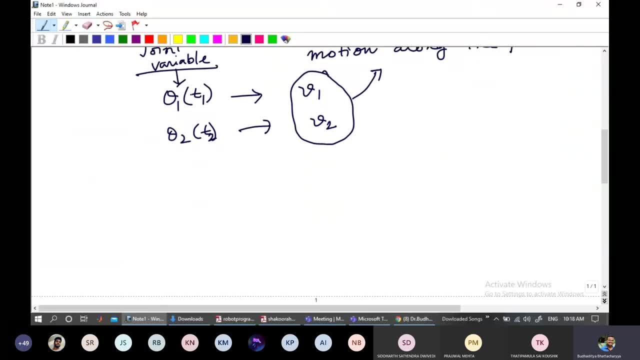 Now, just to give you an ideally a scenario, that where does this come? this path planning comes in, so maybe I will just give you a small little flow chart of it. so maybe, like, this is the process, like we have a task. ok, everyone is following this. 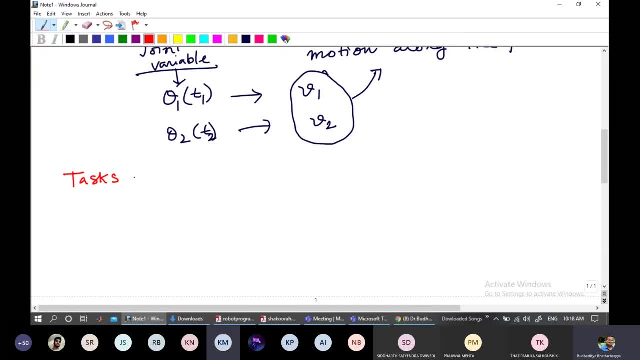 Everyone is following this. finally respond: yes, yes, sir, yes, sir. ok, so this is my task. so any task we have, whatever the task we have, we are processed. now we have to have some kind of a task planning that we have to go now. what is task planning like? maybe we can. 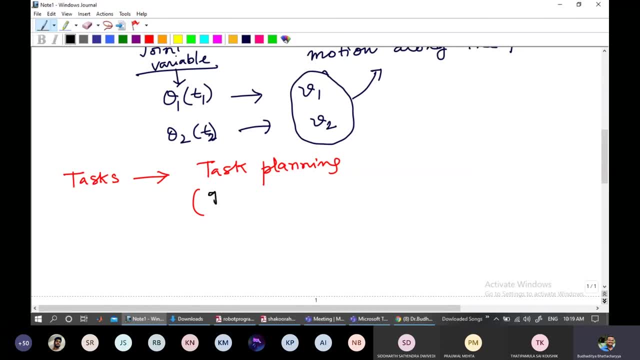 say, the task planning includes: go from one position, go from one position position to another. Ok, So this is what the planning is. so to this is what the task planning is: one into another, ok, so this is what we already did. now, after this, after this, the path planning comes in. 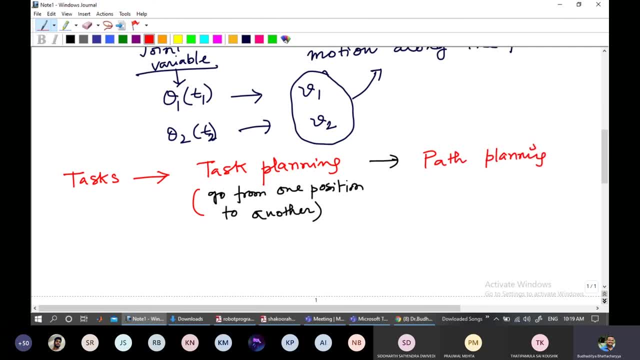 that is how to reach. ok, so just to give you an understanding on path planning. so this is nothing but some set of points, as we had already discussed. so this is some set of points, so we will specify some points through which it might traverse the same path. 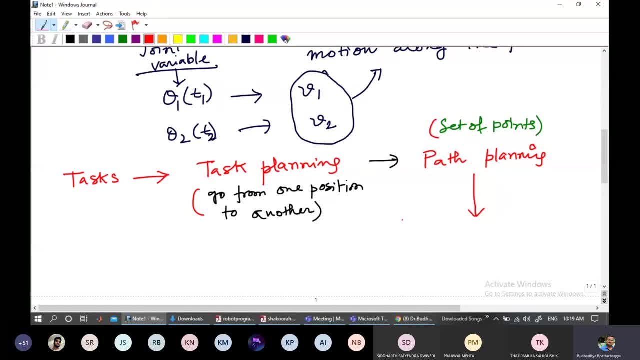 Ok, And naturally, after this will be the trajectory planning that will come. ok, so this is what the idea behind the trajectory planning is, ok, So so trajectory planning, we have this as based on, based on the set of points, specific, specific planning data That needs to be done. and after this, when we are looking at this, is where the controlling 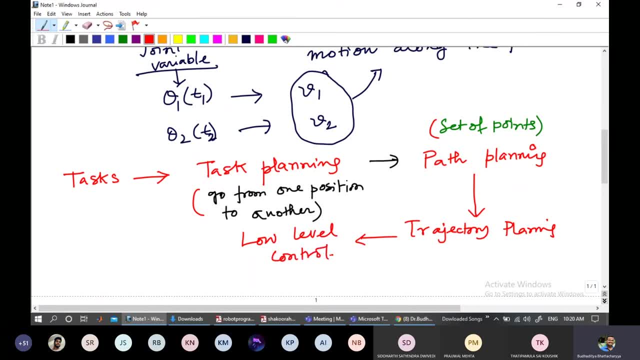 action will come, So low level controlling will come somewhere over here, that how we will control it and finally, the output will come over here. ok, So based on this scenarios, you can observe that this is what we are trying to specify over here, or we are of our interest. 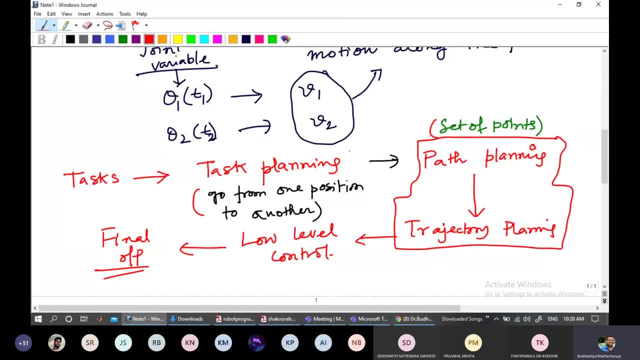 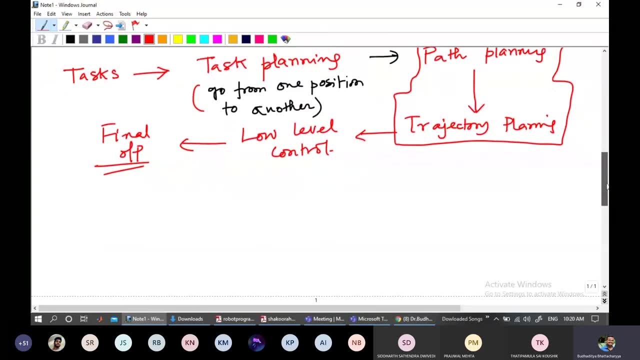 This task planning is nothing but the forward and the forward kinematics or the reverse kinematics that we have studied, And this is what we are going to study now. ok, Now let us see how we are going to do it. just take, take this small example to understand. 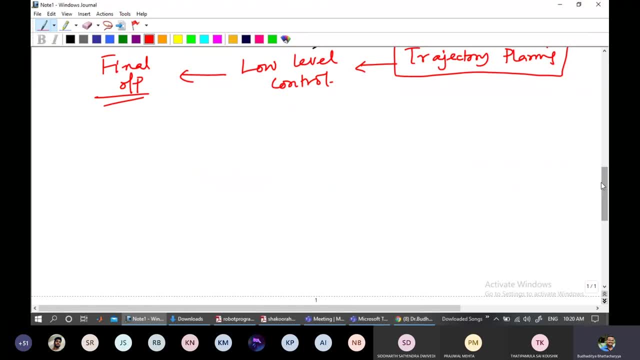 that? what is the role of the task planning? let me take this small example. So suppose I have a two dimensional, we have a very small conventional 2D plane. suppose we have something like this: we have an x over here and we have a y, so we have a joint somewhere. 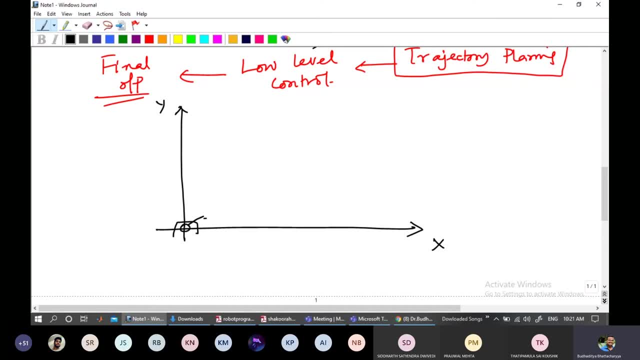 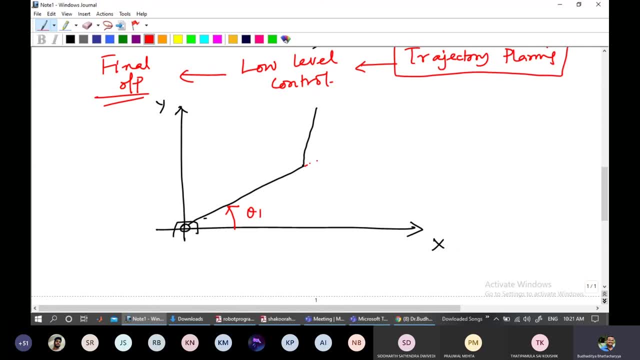 rotational joints is theta 1 and we have something like a theta 2 over here. So what it does is that we have a starting point- s ok- and we have a destination point, maybe somewhere over here, which is go like g- g point over here. 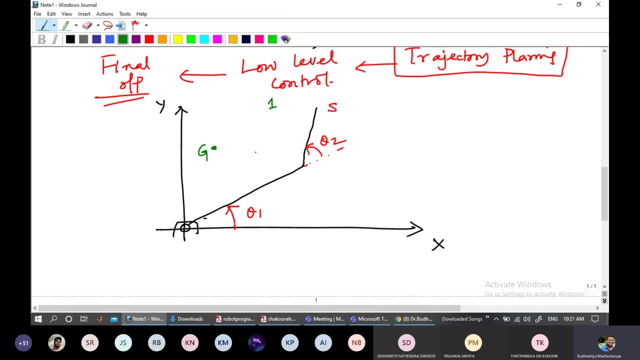 So what we are looking at that through this point- 1, 2 and 3- maybe this way, what it will do is it will go. this point will go something like this: So this is the point, it will move. ok, Now you can observe this. 1, 2, 3 can be any point, but this is just for our clarification. 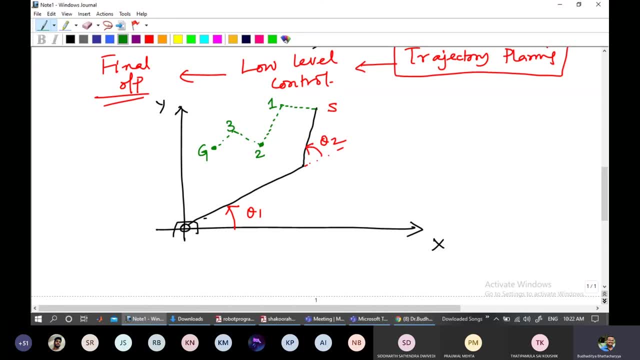 We are just making sure that there are three points through which it is passing through, ok, and this is the overall nature of it. So this is my source point and this is my destination point and these are the inter between points. ok, Now, theta 1 and theta 2 being the joint angle, we can represent this in terms of something. 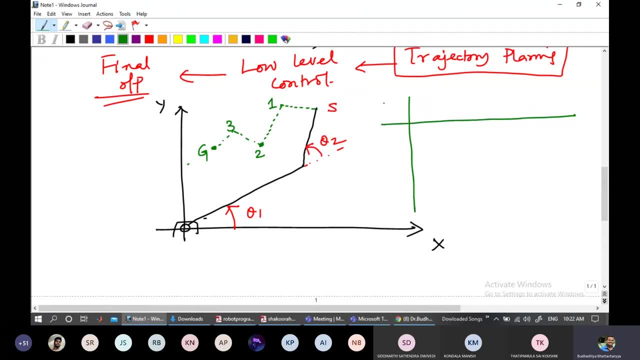 of this nature, which is quite obvious. So we call this as the points, We call this as the task space- Ok And space. Please make a note of this task space and the last one we call it. the next page is joint space. 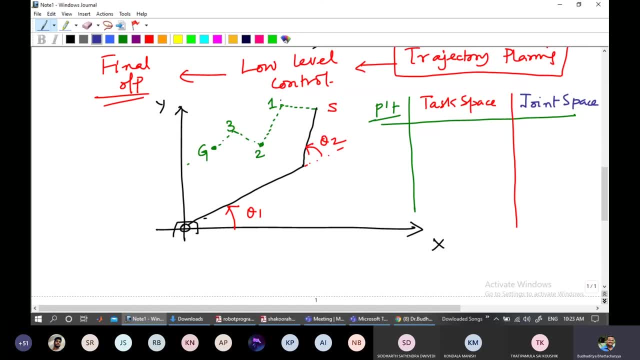 So what is this two space? I will explain one by one. So it is at the starting point. So the point is s the task space will be nothing but some coordinate that is in Cartesian plane. Ok, So this is my x s and y s, and I will mention theta 1 s as the joint space and theta 2 s. 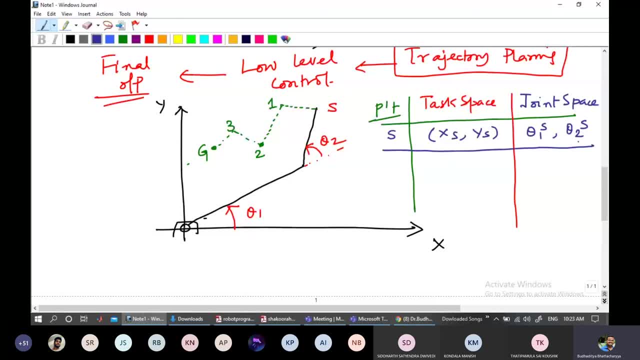 as the starting point, joint angles. Now, when it is at point 1, when it is at point 1, this becomes x of 1, this becomes y of 1.. Similarly, theta 1: 1, theta 2: 1.. Ok, So this is my x s and y s, and I will mention theta 1 s as the joint space and theta 2 s. 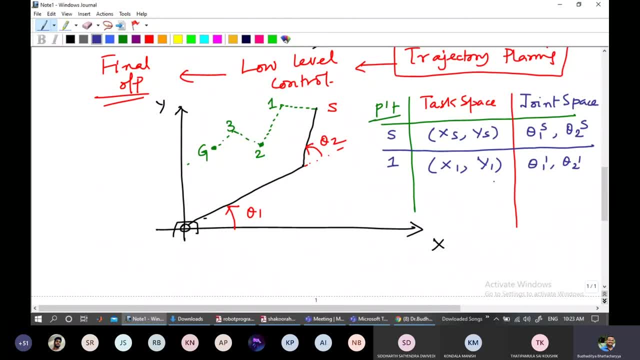 as the starting point, joint angles. Ok, Then again we have second point, which is x of 2, y, 2, theta of 1, 2, theta of 2, 2, and goes on till the point g, the last point g, which is x of g, y of g and theta of 1, g, theta of. 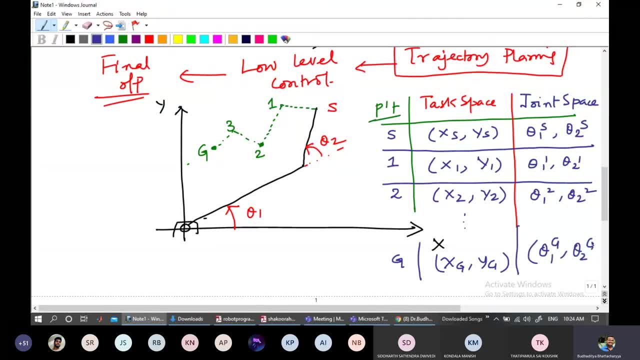 1, g. Ok, So this is. this is overall, the process. Now, to be honest, there are two ways. there are two ways in in which we actually can make this calculation work. Ok, So now you can. also. this is the path: this s to 1 to 2, to 3 to g. this is what the path. 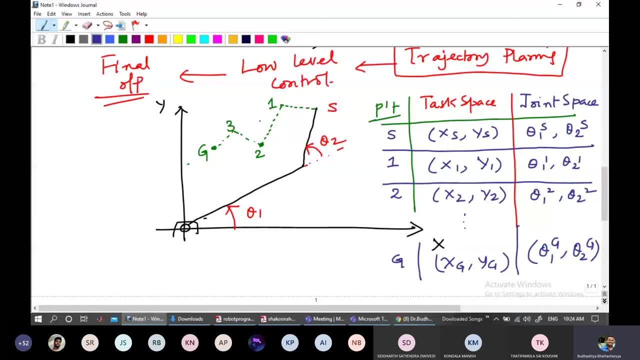 planning is all about Now how this path will look. something like this It could have been. it might have looked something else. maybe an arc could have been here and we could have come from s to g. So what? whether we should choose that arc or whether whether it should be a linear part. 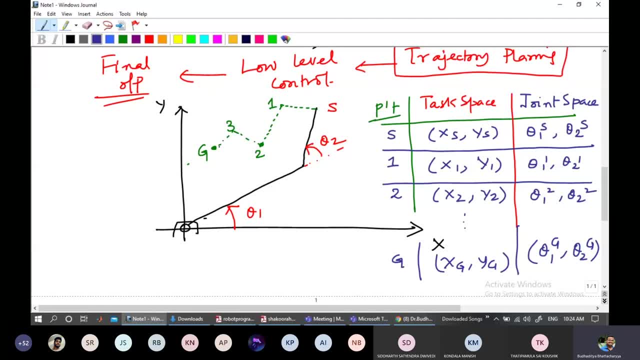 or whether this should be a zigzag like this. all this is part of the trajectory planning, and the points that you are referring to as 1, 2, 3, this comes under the path planning process. Now, this calculation of this can be done either in task space or joint space, that is, either. 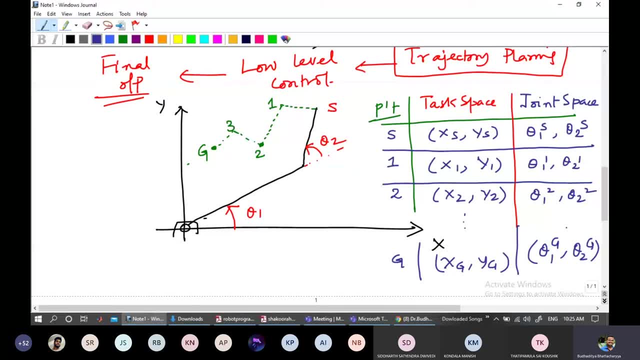 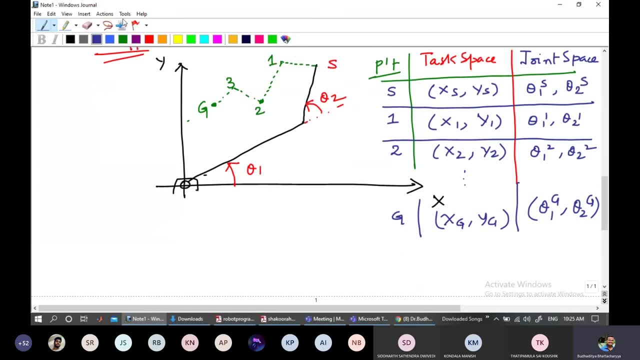 in the Cartesian coordinate plane or in the revolute plane or the rotational plane, but ideally it was. However, it has been observed that this calculation under this task space- please make a note of this- that calculation, calculation in task space, which is the the Cartesian plane, we 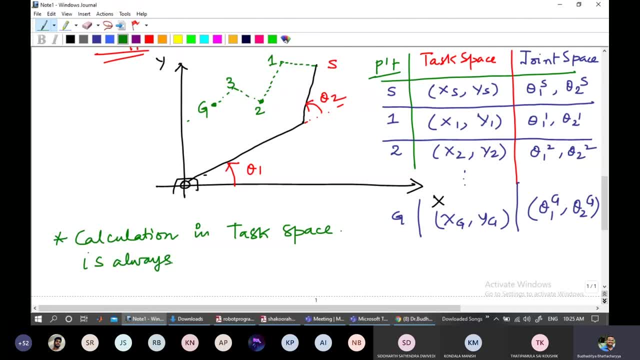 are talking about is always difficult, is always difficult as here inverse kinematics is involved. Now, as we all know, that kind inverse kinematics is always a little difficult. if you remember, just before we ended our discussion, before the the shut lockdown, I told you that we had 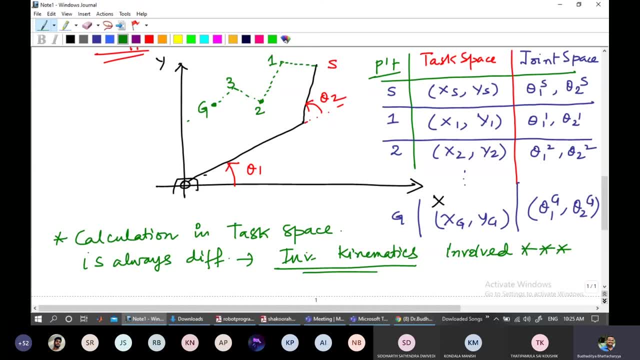 gone through a class on inverse kinematics as well. if you can go through the video which I have uploaded based on that, you can find that. So, for inverse kinematics, what happens? that, given a set of points in the other plane, we in the, in the in the end end vector, we try to find out what is the theta 1 and theta. 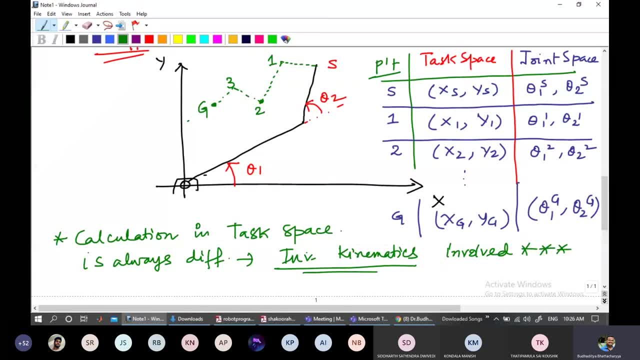 1. Theta 2, inverse. and that calculation, the inverse kinematics problems are always very difficult, So it is computational challenge, computational challenge. and when you try to do this inverse kinematics for a given robot, for a very complex robot in fact, and when you try to do that, 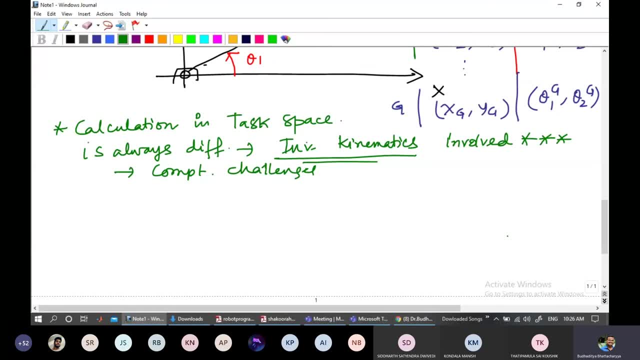 on the go online like real time. if you are trying to feeding an inverse kinematics, it's always a difficult task And that is why That is where the joint space calculation is always paper. joint space based calculation is always preferred for path planning. Please make a note of this, that we always have to find out that. what is the joint space? 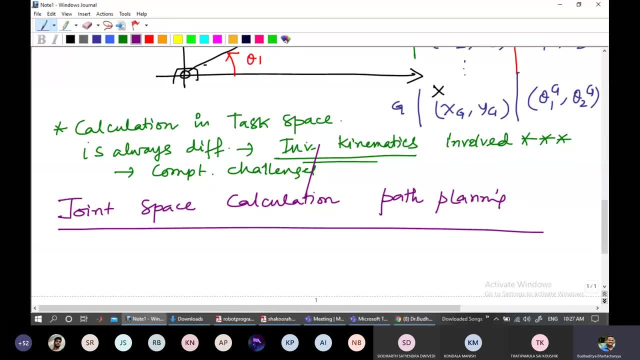 we have to ensure that there are joint there. there are the joint space, how the joints are moving and based on that we have to make sure there is a continuous movement of the of the joints such that we can figure out that what are the nature of path that it will follow. 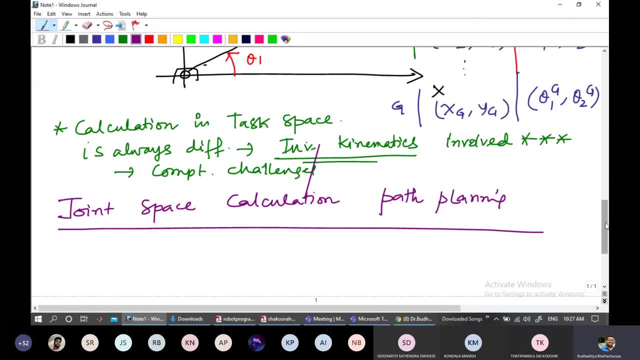 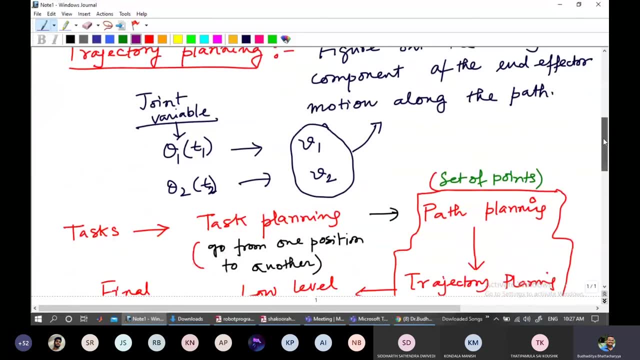 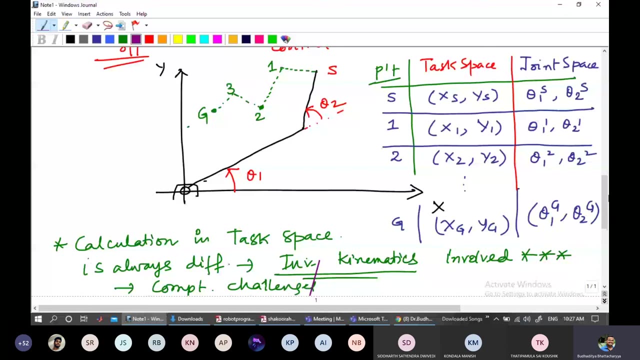 So, based on this, any doubt till this point, any doubt till this point, people, Can I ask anyone a single simple question? Can anyone answer me? what is the if? suppose I want to have this particular diagram, if this diagram exists and if I want to change? 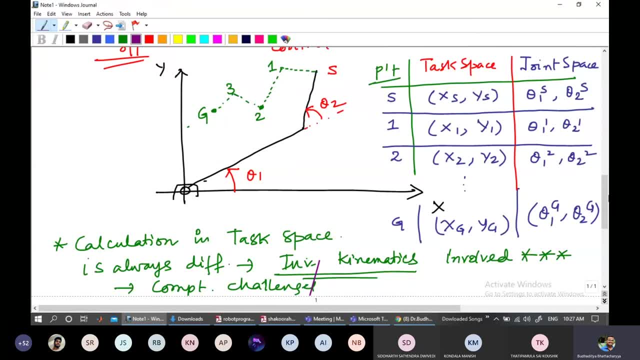 1,, 2,, 3 as the three different points. will that be considered as a trajectory planning or will it be considered under the path planning? The question is: we have this particular diagram. Yeah, Anyone. please introduce yourself and then answer the question. 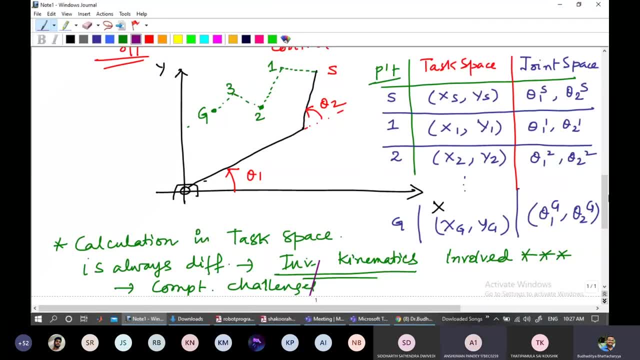 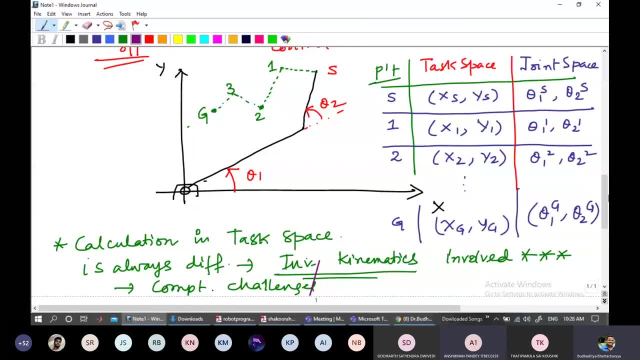 uh, so anshuman. your registration number is uh 17bec0259. okay, so, uh, uh, in case of uh, path planning, this is path planning in fact, because when you are changing the points from one, two, three, it can be any points. in fact, it can be any point but based 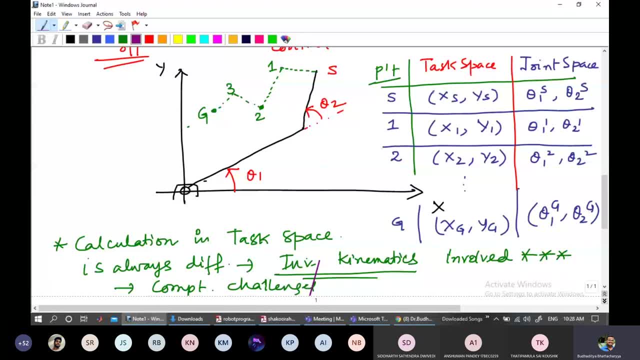 on the requirement, we can fix the point through which it can pass, because it might happen that this one at point you need to pick up something, you need to pick up something over here as well, or you have to drop something over here, and then maybe you have to collect something over here and 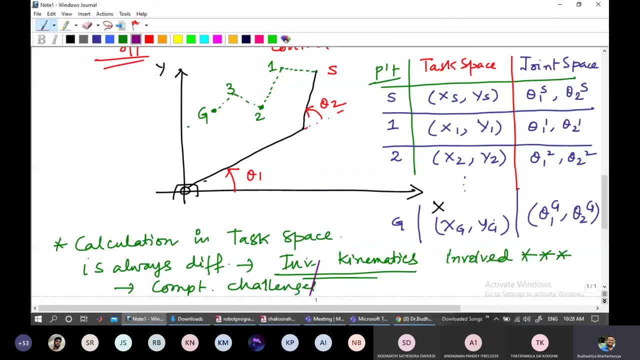 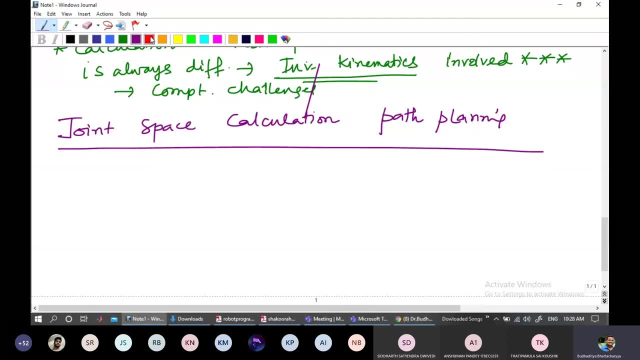 you have to put it over here in g. so, based on the requirement, we will go on changing the uh path, for that matter. now to ensure uh- this is very important, in fact, the two points that i'm going to write here, so to ensure so- we are also confident that joint space calculation is much, much easier. we'll 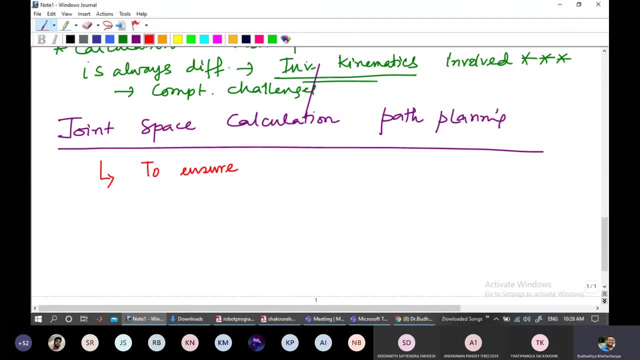 see that, in fact, that it is much more easier to find out using joint space rather than the cartesian plane because of its inverse kinematics, that is involved with the calculation. so to ensure this smooth, the smoothness, the smoothness of the joints, because there should not be any jerky movement, because if you are suppose you 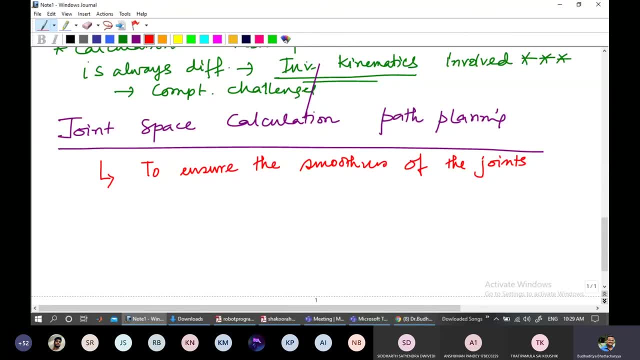 are picking up something. so there is a velocity that is involved with the arm- robotic arm- that will go and pick up something. so if the velocity of the arm is not continuous, okay, if the manipulator is not continuous, if it is not smooth, then naturally there will be a jerky. 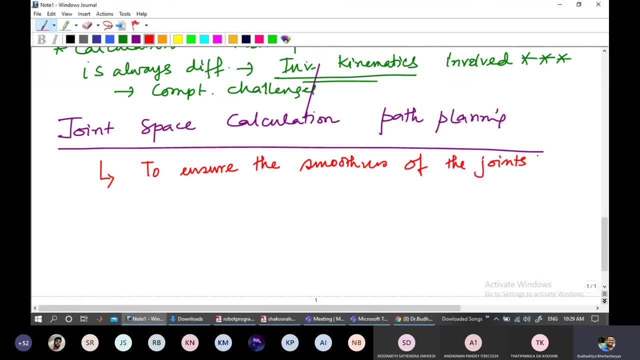 movement that will be associated with it. so we are not, we, we don't desire to have that actually so, to ensure the smoothness of the joints of man, of the joints in a manipulator, in a manipulator, the angular velocity, angular velocity, okay, and the angular acceleration, and the angular actually see angular. 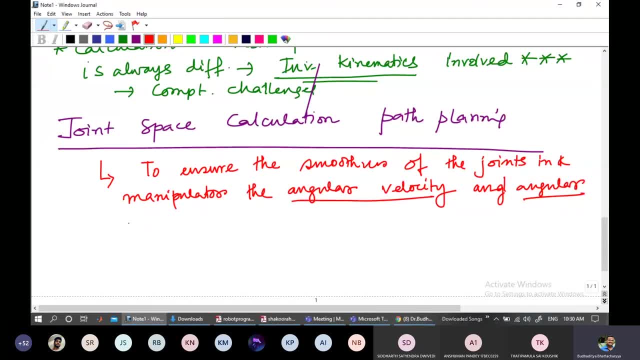 acceleration, angular velocity, because it's a rotational thing that we are considering, that we are looking at. so the angular velocity and angular acceleration must be counted okay, because this is what the idea is, because if we can get hold of the velocity and the acceleration, that would happen to an end effector or to the manipulator at 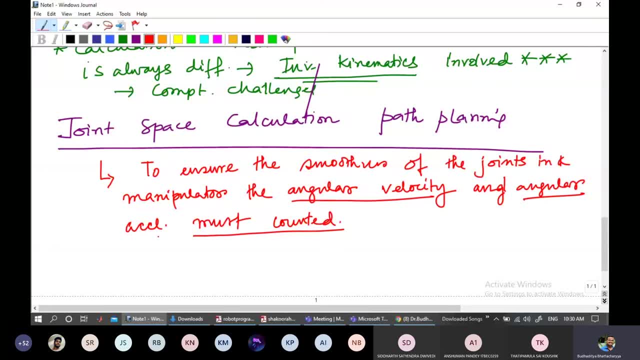 a given point of time we can find out what is the smoothness or what is the nature of the movement or the path that we are following. So jerky motions are not desired, as I said, because it may definitely cause vibration and maybe wear and tears, and on the manipulator as well as the object. 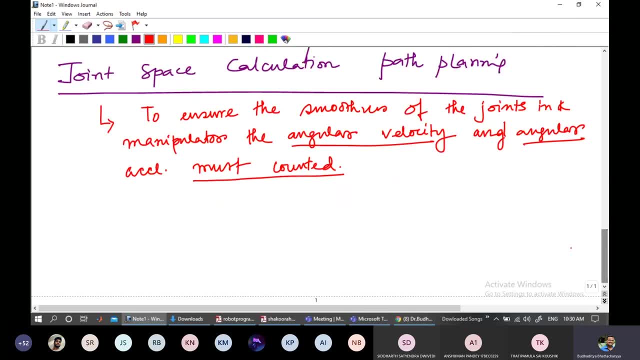 that it is going on picking, So the primarily there are few techniques. that is usually used for this process, So we directly go to some common trajectory. So whenever we are considering this angular velocity as well as the acceleration, this is where the trajectory comes. 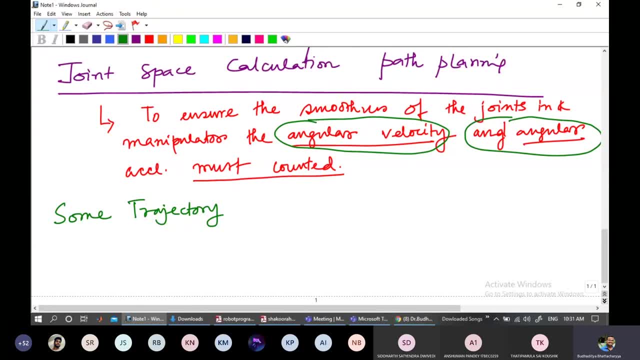 in. So now we are mixing both the path planning to the trajectory planning, because we are now going to involve the angular velocity and angular acceleration to the equation, So the some trajectory function that we are going to look at. So the first trajectory function, 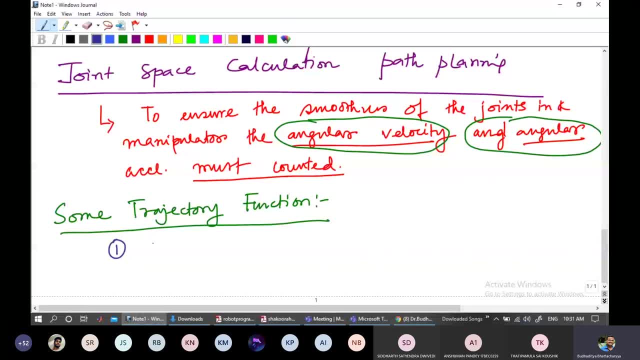 that there are three primarily. So the first thing is called as the cubic polynomial. very easy in fact. we will see that one by one. The second one is called the fifth order polynomial, or we call it sometime as a quintic polynomial. fifth order polynomial. 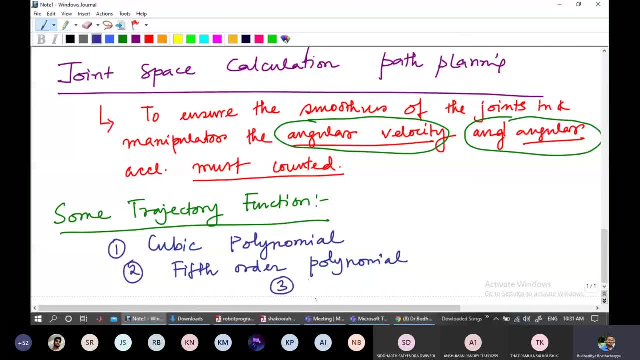 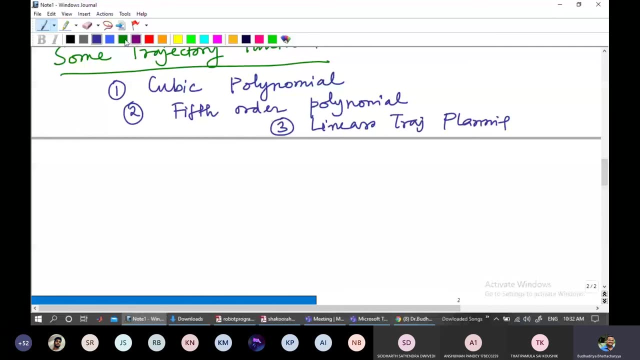 and the third one is called the. this is a different part, although linear trajectory planning. We will see this next, this linear trajectory planning, separately sometime later. So let us first discuss on the cubic polynomial, because this happens to be the most discussed topic in this particular segment. So let us see how it is made and what is this all? 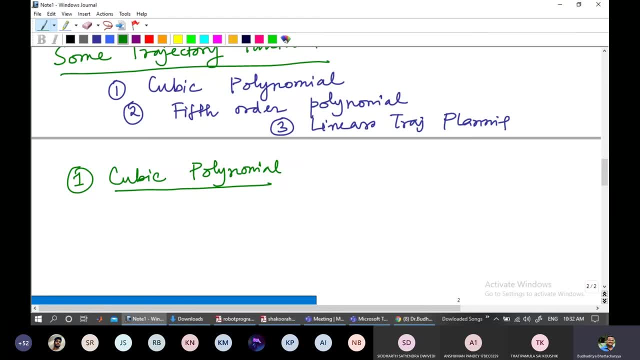 about. So if suppose so, by this time we are sure that the arms or the end effector of manipulator is moving from one point to another, based on some desired path. Also now for the timing. we have also included that there is an angular velocity and angular acceleration that is placed along with 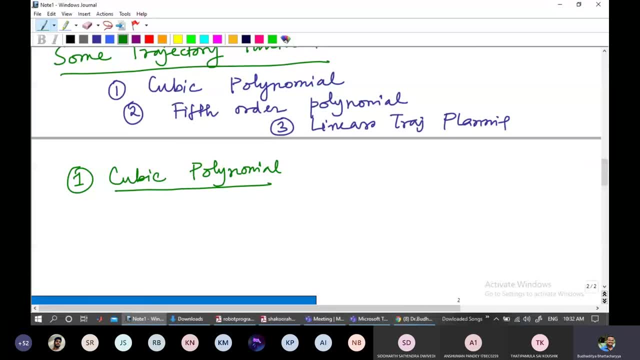 the motion, along with the arms that we are looking at. So suppose we have a scenario for we call it the first, Case 1, where the conditions are the initial- please make a note of this- initial and final values of joint angles. that is theta, Suppose it is known to you. we want to find a continuous 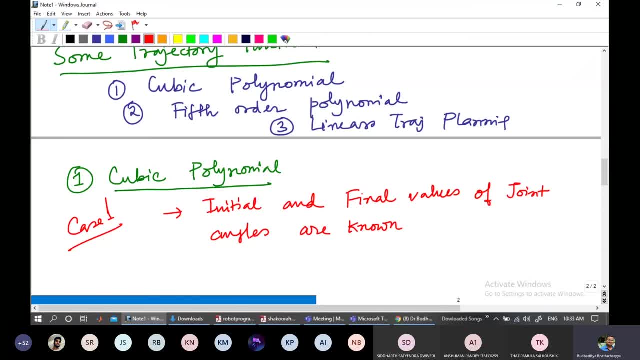 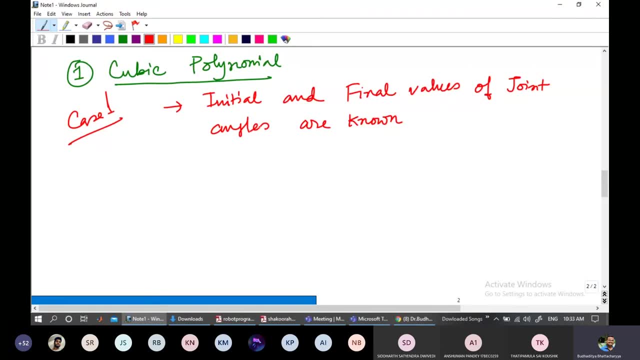 polynomial equation. Okay, that we can find out what is the nature of trajectory it will follow. So initial and final value. suppose this initial and final value of the joint angles are known. So theta is unknown to us. Next is the angular velocity at the beginning and at the end. 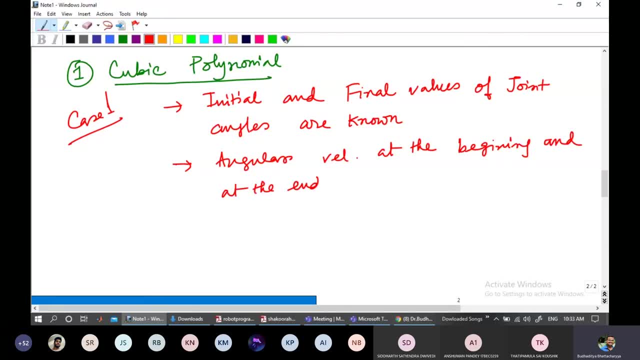 And at the end of the cycle are kept at zero. This is the most used process, because you can observe that what we are talking about in the second point, This case one will be referred many times because some numericals will also come in with respect to this particular condition. 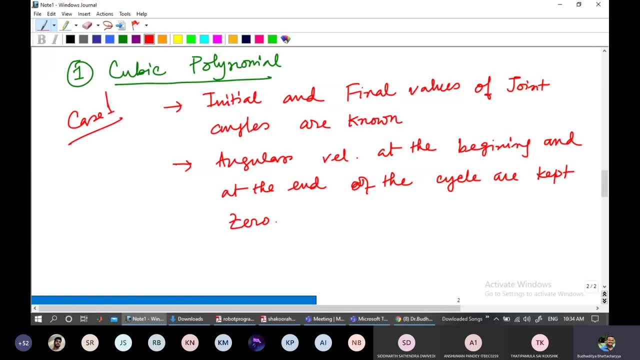 You will soon find This is very simple, very easy In fact. we will see that one by one. So the two conditions you just observe: The first condition is that at time, t equals to zero, if I call this as the initial. 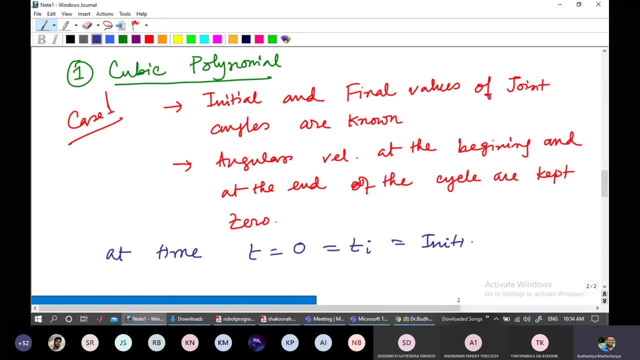 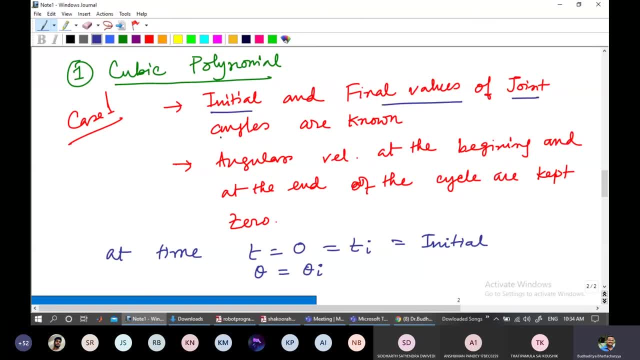 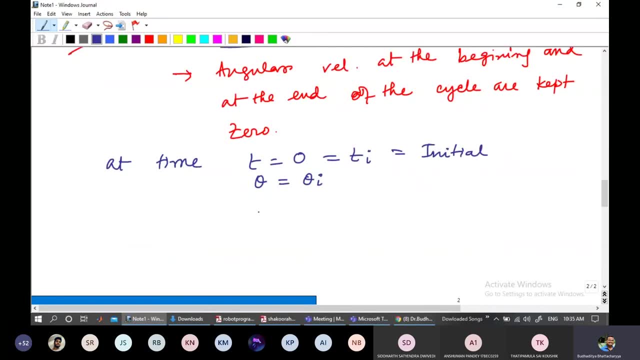 So this is the initial time t i. So this is the initial time t i. So this is see that initial and final values of the joint angles are known. So the first point is theta is known to us. I will see that I will try to draw another diagram along with it. 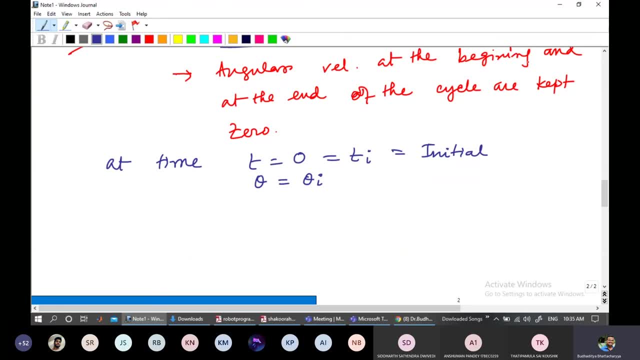 And also we can observe that second point condition: angular velocity at the beginning and at the end. at the beginning and at the end of the cycle are kept zero. So we will write this way: theta0 or theta prime, that is equal to 0.. So this is, these are the 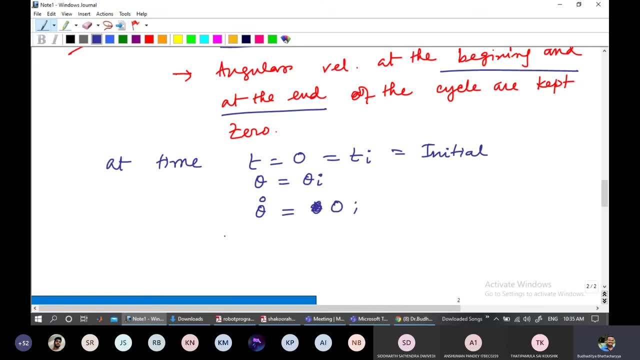 conditions which are there. Now we are going to see. let us simply make a неё cycle and we will look at that. The second point that we are going to see is that, at the beginning and at the end, This is the. these are the conditions that we are looking at. So at time, at time, t equals to t f. 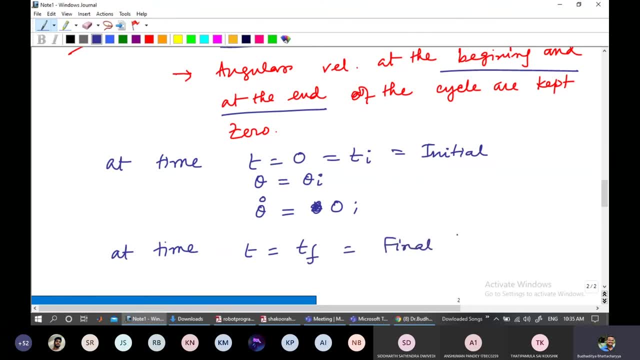 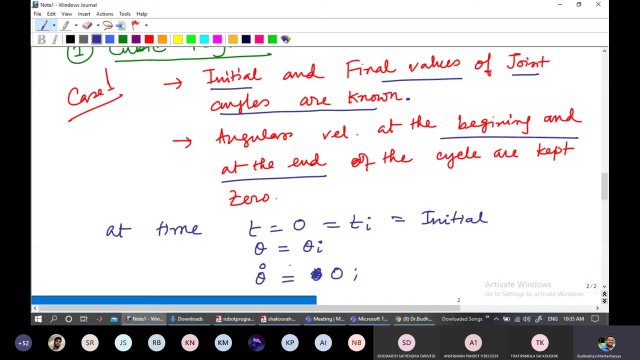 which is the final time that is. So this is the condition. final time. theta equals to theta f and theta prime is is 0 once again. So see this two condition I have. I have mentioned it over here that the initial and the final value of joint angles are 0.. So this theta i, maybe you. 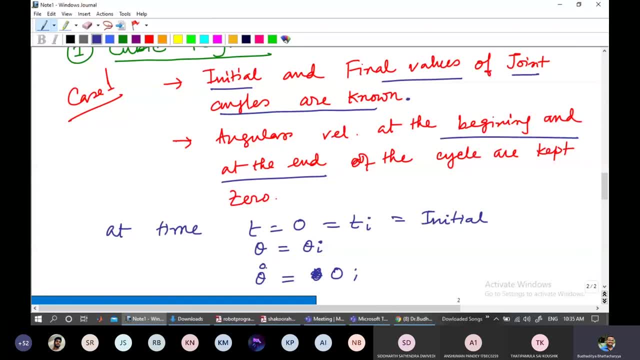 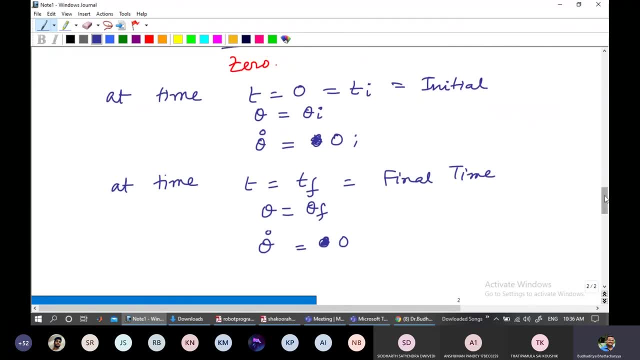 can write it as theta. i prime as well. So, anyway, leave it. So theta dot is equal to 0 as well. as you can see, at the final instance also, theta is equal to 0.. So now we, we want, to want to. 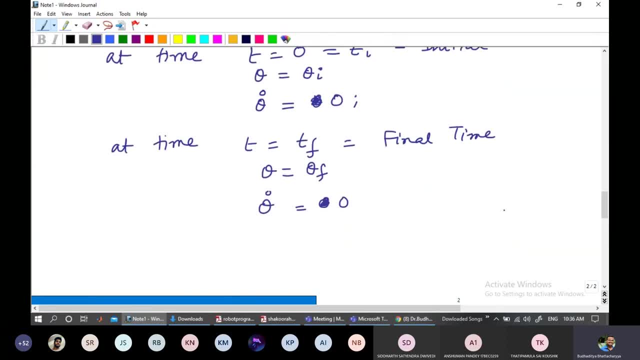 categorize this condition into a polynomial, into a polynomial equation, for that matter. So what are? what are these? So let us, let me just write it once: The order of polynomial. please make a note of this. the order of polynomial is determined, you will see it. it should not be clear to you what I am trying to do. 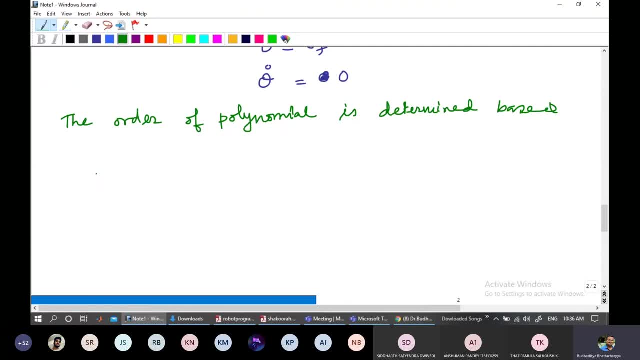 So the order of polynomial is determined based on the number of boundary conditions. This is pretty interesting and important boundary conditions. So this is pretty interesting and important boundary conditions. So this is pretty interesting and important boundary conditions. Please make a note of this. 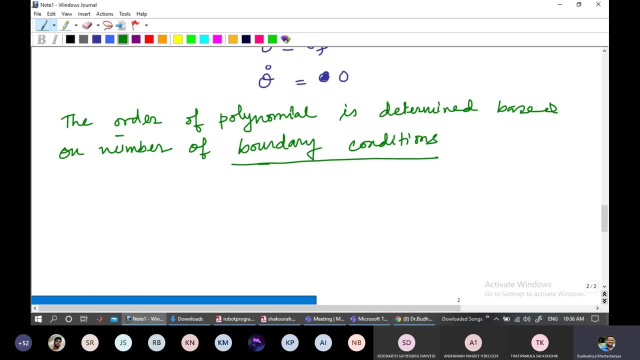 Please make a note of this. So we will form a polynomial, the order of polynomial based on the boundary conditions given. So if n number of boundary conditions are given, ok, then the order of polynomial. order of polynomial should be n minus 1.. Please make a note of this. It is very important because based 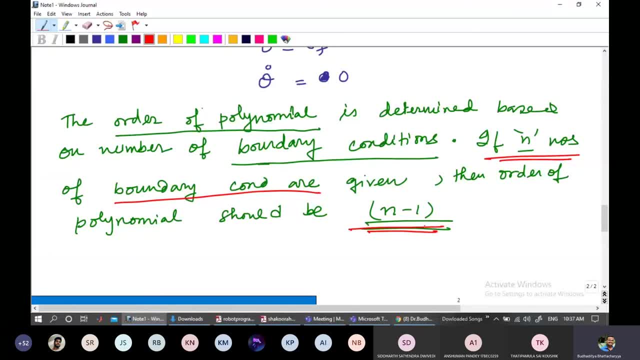 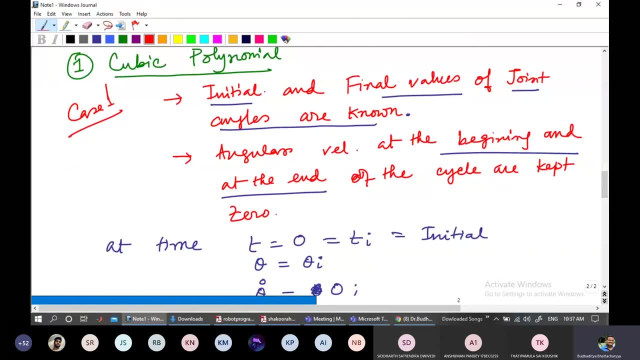 on this only you can solve the questions. all the numericals associated. So here you can observe. for this case we have four boundary conditions. If I go back so you can see the first two boundary conditions is on the angles. So initial and final values of the joint angles are known. 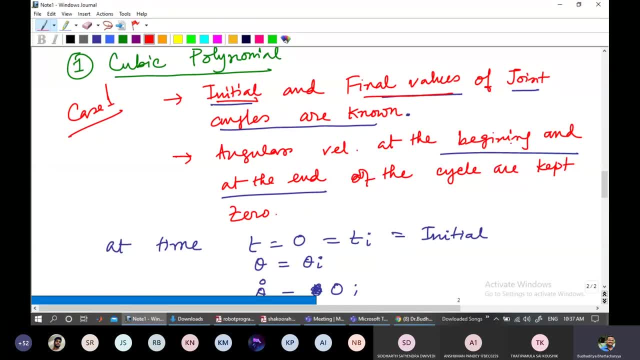 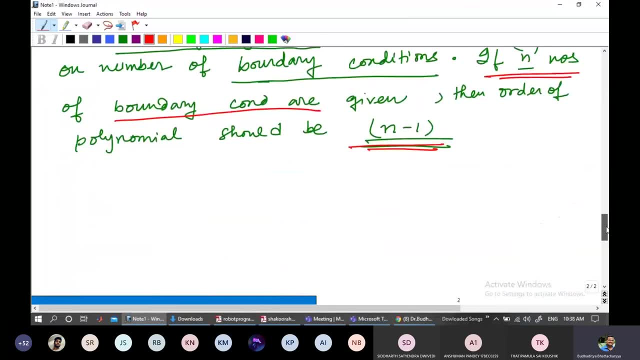 So this is two boundary conditions. and angular velocity at the beginning and at the end of the cycles are kept 0.. So this is another two boundary conditions. So basically you have four boundary conditions here. Hence my polynomial equation will be in the order of: 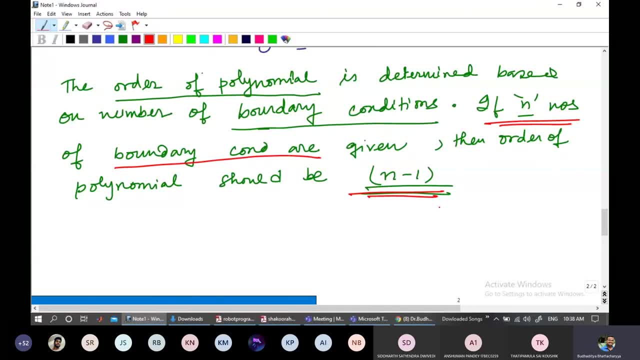 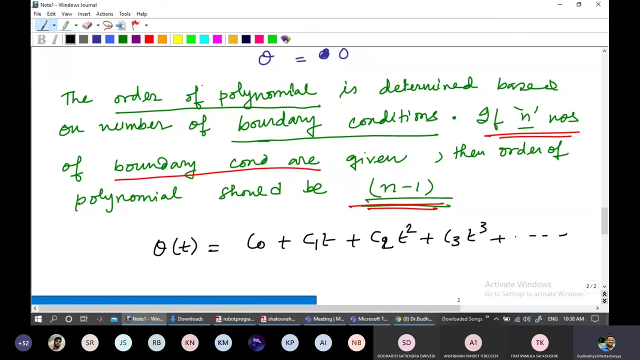 three degree polynomial or a cubic polynomial. Any doubt with this? Please respond. So what I can write in general, The generic equation should be C0 plus C1, t plus C1.. The generic is something like this: C2 square plus C3- cube. like that it will go on. This is a generic. 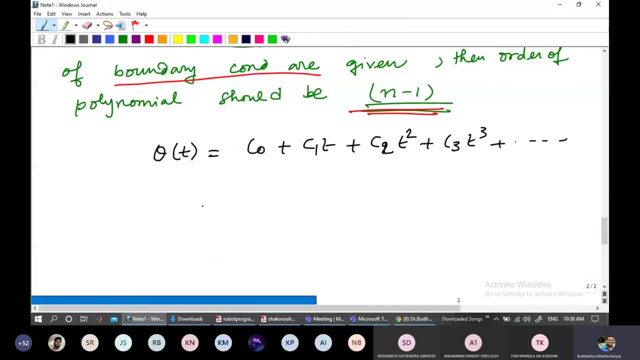 equation. but for the specific cubic polynomial we can write theta t as only C0 plus C1, t plus C2 square. So this is my generic trajectory: cubic polynomial based equation based on four given condition or four given boundary condition for us. So please make a note, This is my. 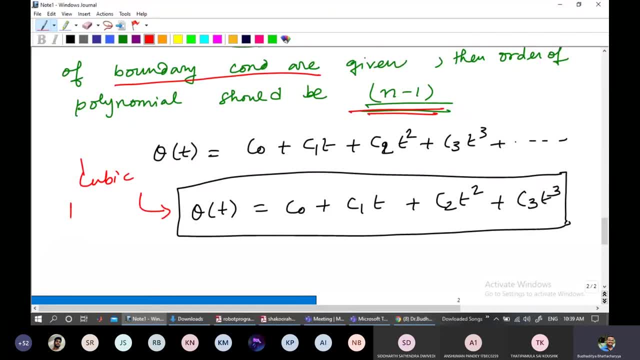 cubic polynomial that we are going to refer all throughout. Why this is important? Because in most of our numericals that I have come across and the most of the condition that we refer to, you have to remember that the cubic polynomial of any given integral is equal to a constant of. 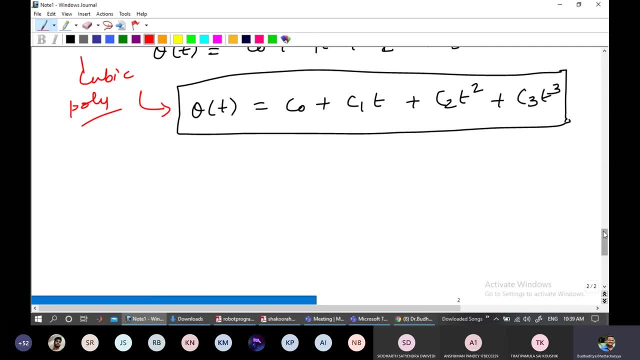 theta. So, again, this is a very common example. This is one very common thing that we are following. Just to give you an insight-just to give you an insight- on what exactly I'm talking about-let me just draw a diagram. Ok, let me just draw a diagram on this so that it is clear for you. So maybe I'll show you this way. this is my time. Maybe it's not visible that much. This is my time and this is my theta t. 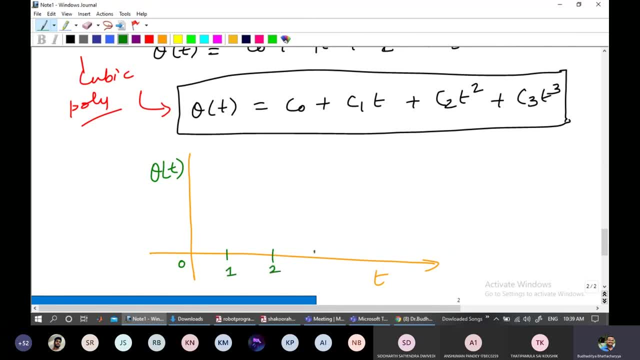 work starts from 0,. maybe this is 1, this is 2, this is 3 and dot dot dot, something like this, and we have certain. this is where the theta i is belonging to. So this is my initial point. 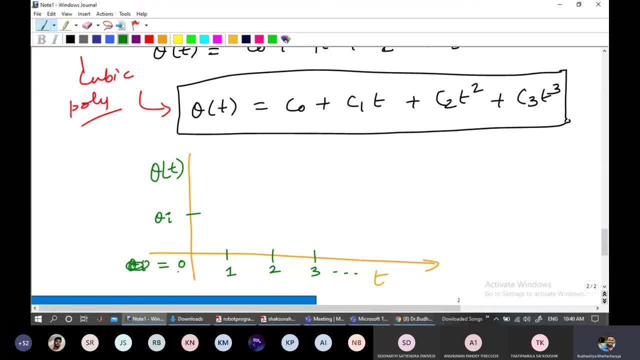 so this may be my theta. i sorry, ti, this is my ti- equals to 0. So at that point we have some kind of a theta and this might be my theta f, So this might be my theta f, for that matter, at some point here, which is tf. So basically we want to find, if suppose this is. 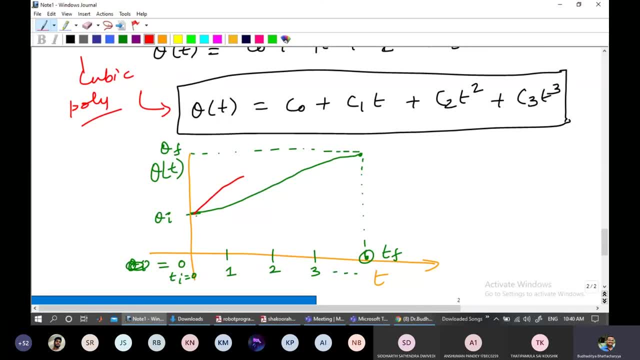 one of the line I am trying to draw. if you are trying to draw something like this, this is also possibility. this can be something like this as well. this can be something like this as well. So the source and the destination is known. we have to find out. what is this particular? 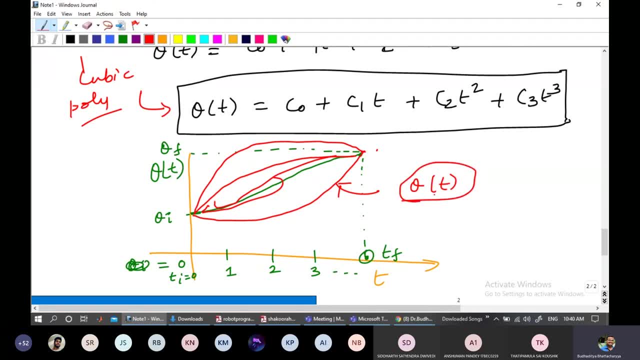 particular path based on the theta t or the cubic polynomial expression. Am I clear with till this point what we did? Please respond back. please respond back. Yes, sir, So this is basically: we are forming a generic equation, a generic continuous time. 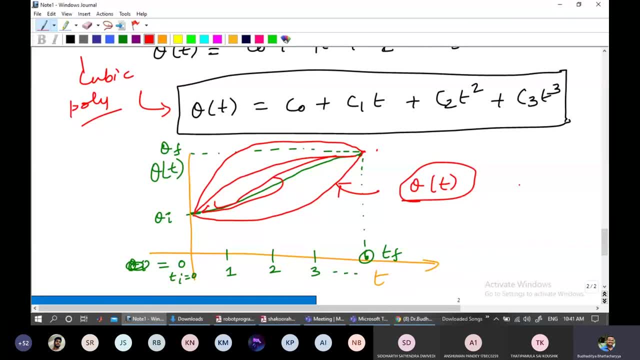 equation so that we can find out that, given a starting and final point, what are, what can be, what can be the trajectory to reach from that starting to destination in a in a particular mathematical way. So this is the equation, So naturally you can observe that the question 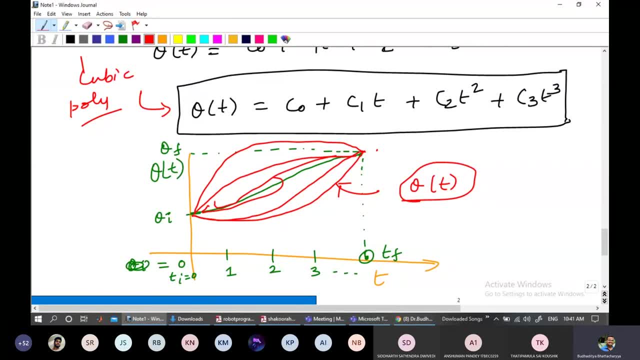 on. this will be based on how to find out this: c1, c0, c1, c2, c3.. So somehow we need to find out this coefficient in terms of the different values of theta and t, such that we can find out. 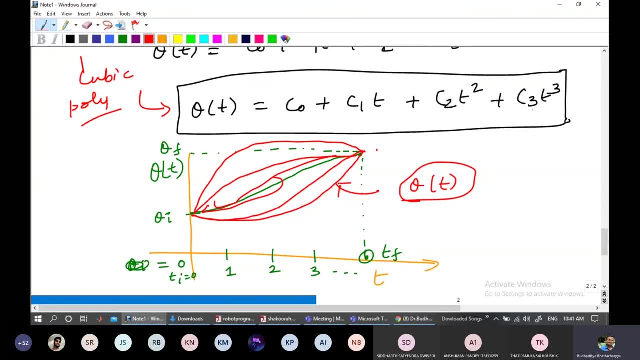 that we can plug in the values over here, c0, c1,, c2, c3, and that will be a generic, continuous equation which might be followed over and over again for that particular manipulator, for that particular condition. that is the initial, initially the angular velocities. 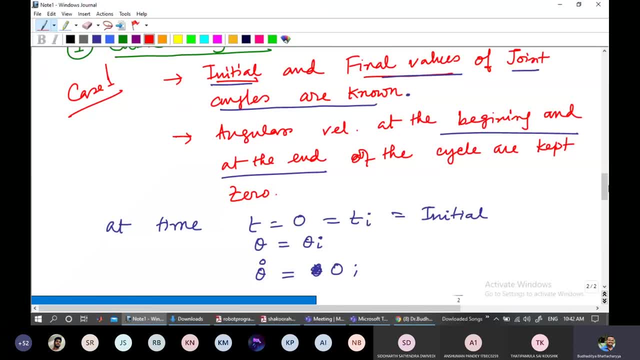 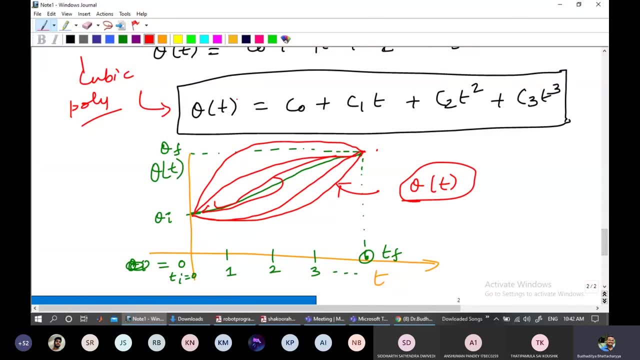 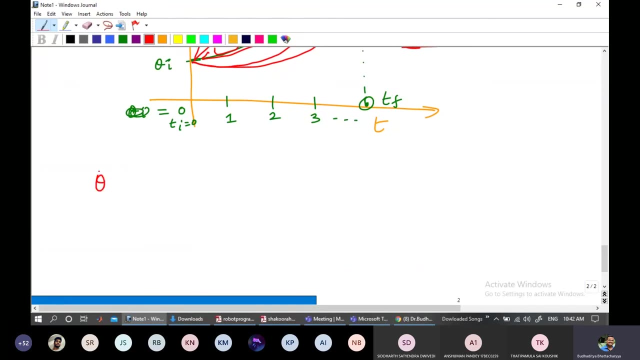 are 0 and at the final point as well, the angular velocity is 0.. Now to consider the angular velocity. we have not taken that yet. this is only the displacement that we have considered, the angular displacement of theta t. So now let us see what happens we had when we are considering the theta prime t. that 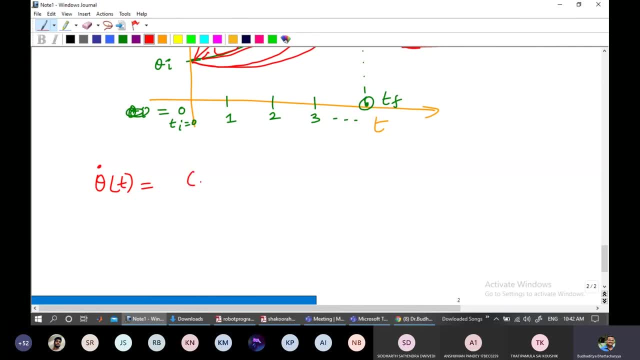 is the angular velocity into the equation. So that will be nothing but c1 plus 2, c2 t plus 3 c3 t square, because, as you already know, that theta t is already given as c0, c1 t plus c2 t square and c3 t cube. So this is all for our reference. So this is all. 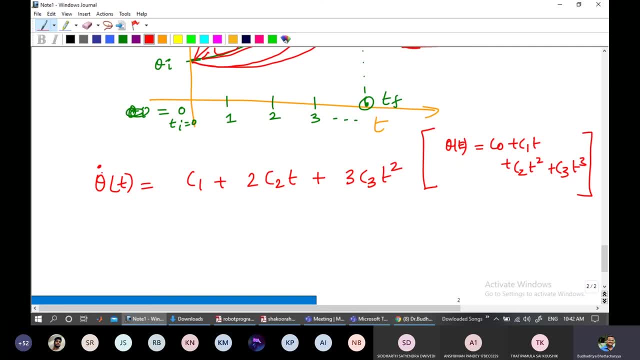 for our reference. So this is my displacement, this is my acceleration, this is my velocity that we are observing. Now let us try to find out one by one: what are these elements, what are these components or the coefficients, how to calculate for this particular case. 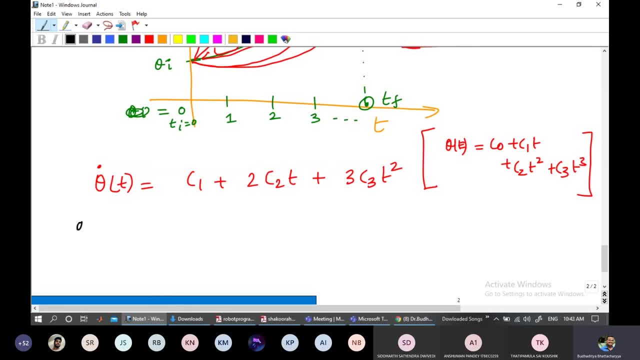 So first is for the very easiest one, please follow this: at t equals to 0, based on the given boundary condition that we have. So at t equals to 0, theta equals to theta i, So we can very well write: So, if theta is equal to theta i, So based on the equation, 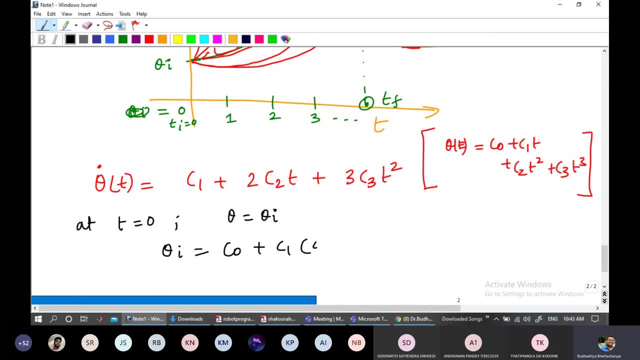 theta i equals to c0 plus c1 0 plus c2 0 plus c3 0.. So this is, if suppose this is my equation 1 and this is my equation 2.. So, referring to equation number 1, we can write this simply: 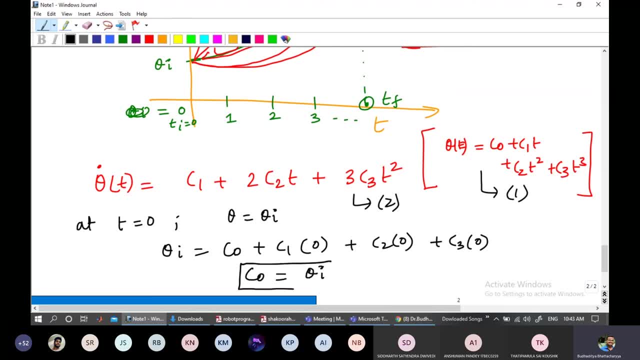 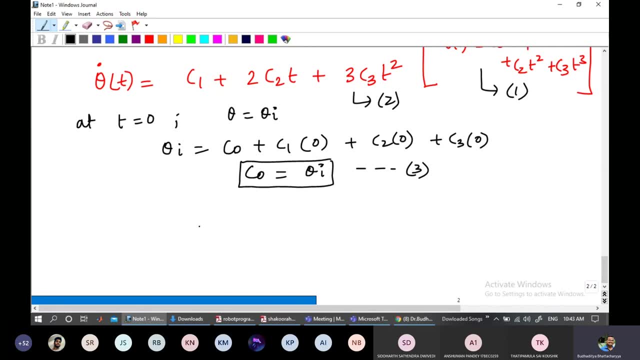 So c0 can be find out, found out by the value of theta 1 directly. So we will write this as equation number 3.. So, based on just the equation and the conditions that we have been given and the same condition, 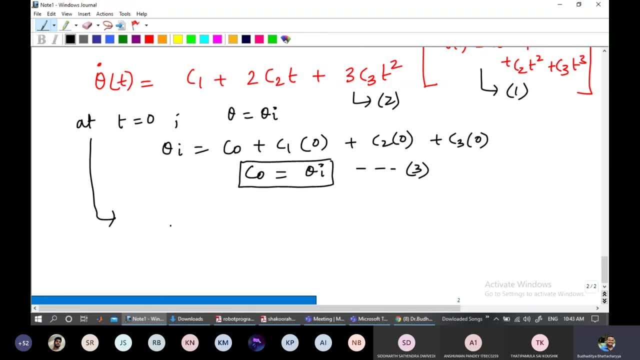 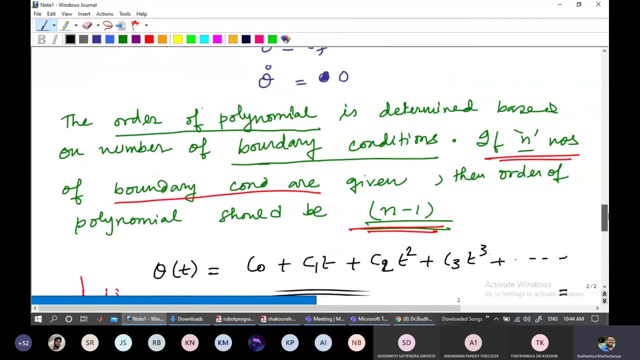 is applied on equation number 2.. So we can write that theta prime is equal to c1. as we are just writing it once again: c2 plus 3, c3, t square Now this is equal to 0.. If you remember the initial: at t equal to 0, the initial condition: at t equal to 0,, at t equals. 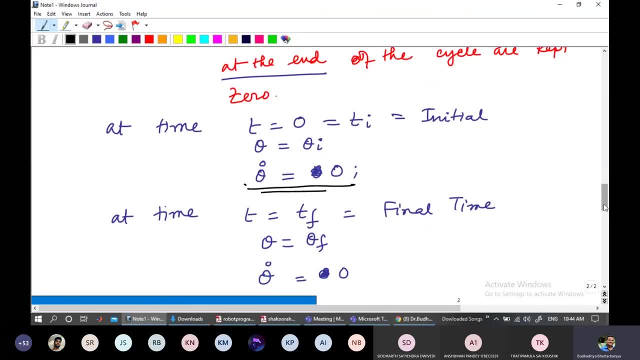 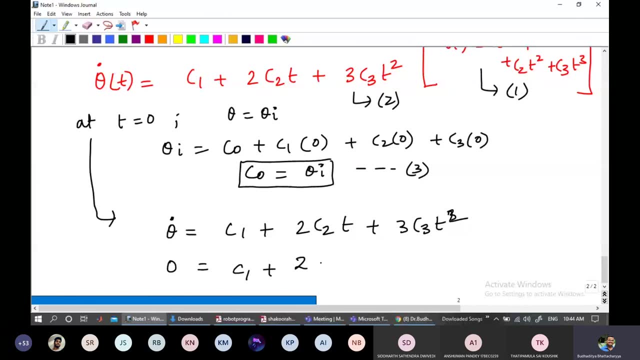 to 0, your theta prime was equal to 0. So this condition, if I substitute over here, so this is equal to 0, equals c1 plus 2 into c2, which is 0 again, because we are calculating all at t equal to 0. So this is what we are getting and that is naturally we are getting. 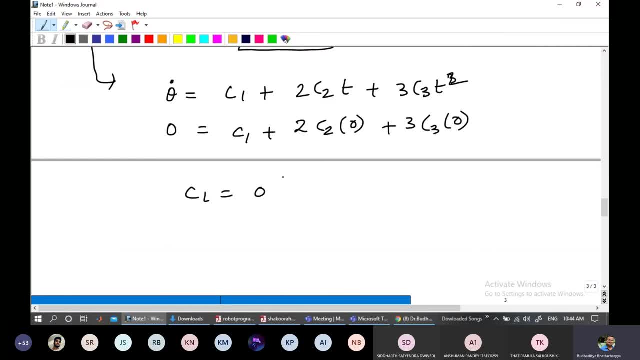 the value of c1, which is nothing but 0 once again. So we are done with. we are done with. that was a very simple problem of a linear regression. So at t, we have taken the boundary condition and we have applied the boundary condition. 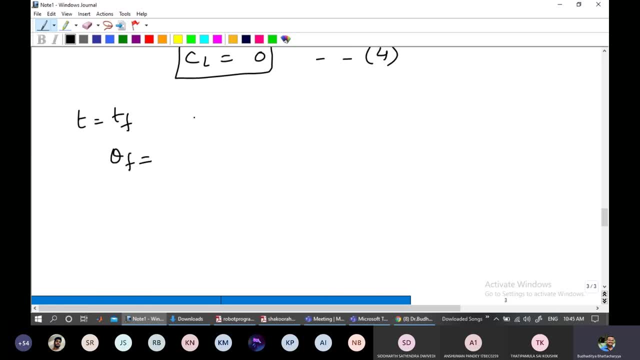 that is the theta prime For this. we are going to write this theta prime as theta prime: c2 plus c1, t plus c3, t square. This is the end of this expression. So we are done. So we have to write that, as c1, c2 is equal to 0.. So now the next step is that we have to find out c1, c2 and c1.. So now we have to find out the other 2, that is, c2 and c3. So for that we apply the second boundary condition. 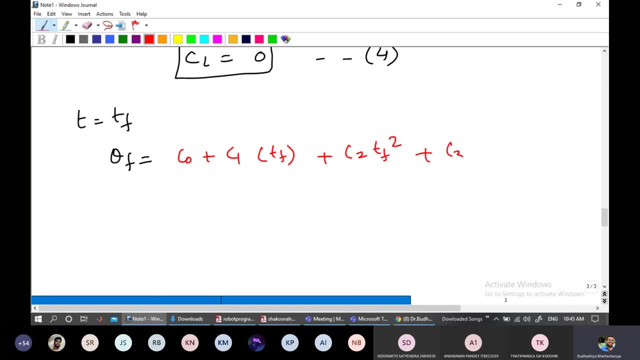 plus c2 tf square plus c3 tf cube, based on the equation number 1 and this, if just this modified equation, we might write it at equation number 5 and from that we can also we can write from the other equation that theta prime f can be c1 plus 2, c2 tf plus 3, c3 tf square, or substituting. 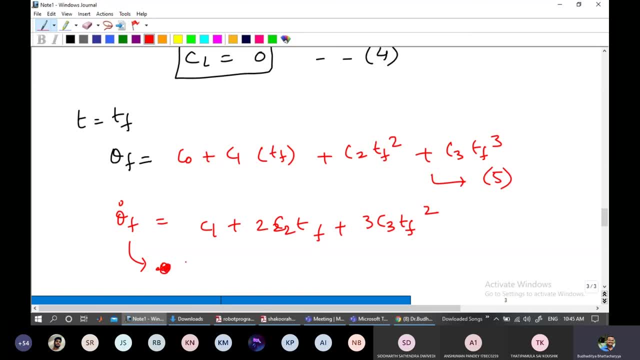 this because initially the final acceleration is also 0.. So the final velocity is also 0.. So this is again c1 plus 2 c2 tf plus 3 c3 tf square, or we can simplify it as in the generic. I am not showing the full step, So it might be: c2 equals to minus 3 by 2 c3 tf. 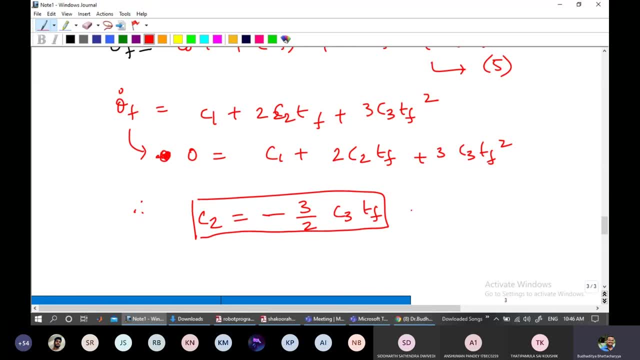 So now we have a condition: after solving it all together, we can find out that, using this 6 equation, there is a relationship between c2 and c3. So by the same process, if we go on calculating another equation, we can find out quite easily that c3, c3, can be find out, found out as 2 theta f minus theta i. 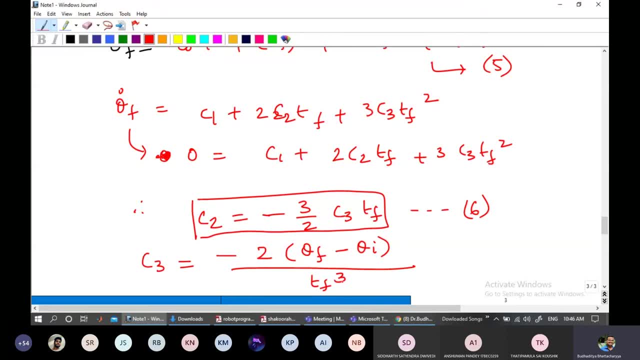 divided by tf cube. It is very simple. you can just the detail calculation is there in my description. So this is a very simple equation. So this is a very simple equation. So this is my in the course material. when I will upload the course material, you can get those. 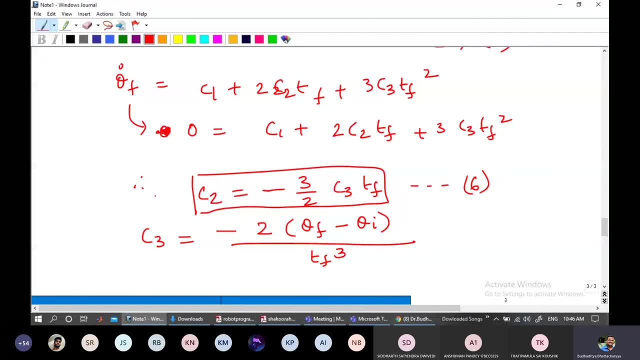 detail. So, for the timing, what we are trying to find out that the c0, c1 is already known, C3. we can calculate in the same manner by substituting the equation, just like in the previous case, and then we apply the c3 on this 6 and we can find out that this is what the idea. 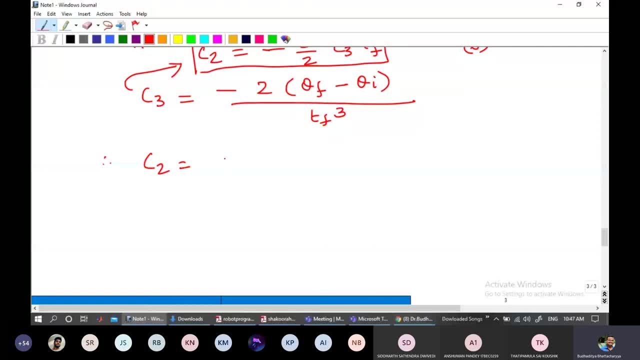 behind. So we get the values of c2 as 3 theta f minus theta i by tf square. So substituting all this we can get the final equation as: theta t equals theta i plus 3 theta f minus theta i, divided by tf square minus 2 theta f minus theta i. 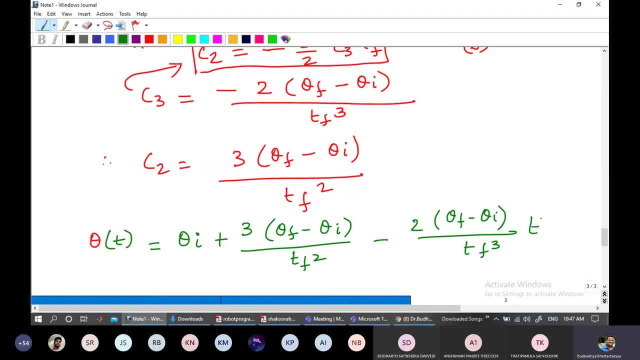 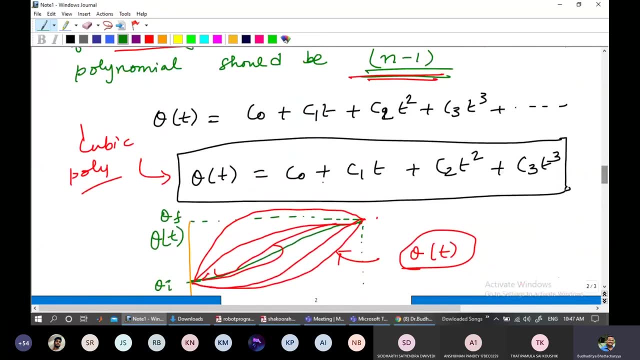 divided by tf cube, t cube, This is t square. So why I written this? Because in the general take equation this was it. So C 0 for us is theta i, So that is why the theta i comes in. 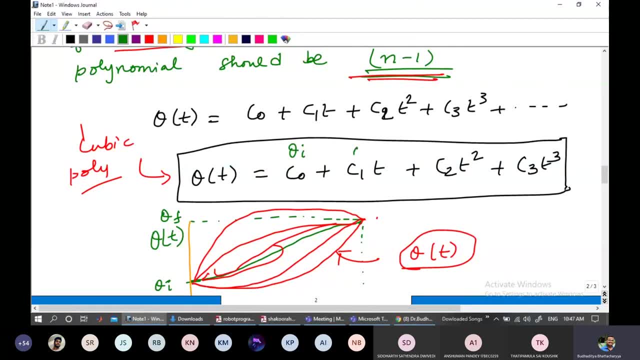 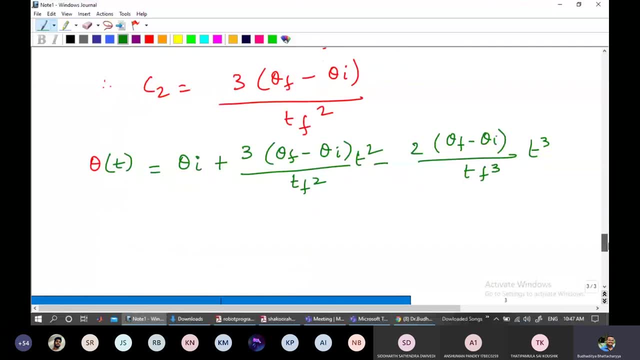 So this is my theta i. C 1 was calculated as 0.. So naturally this will be 0 into t C 2 we have calculated as that equation over here. C 2 is this, So this will be our t square. 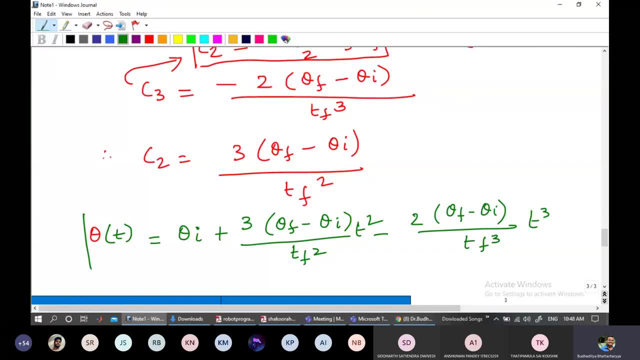 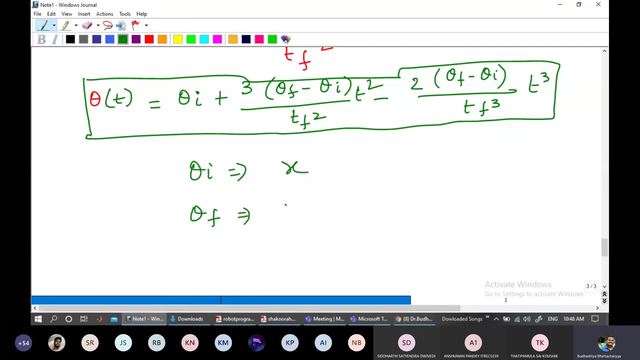 and this is 3.. So minus this into 3T. So this is the cubic polynomial equation. Now, if you can substitute the final and initial theta i theta- i suppose it is x value- and the angle that you want to, 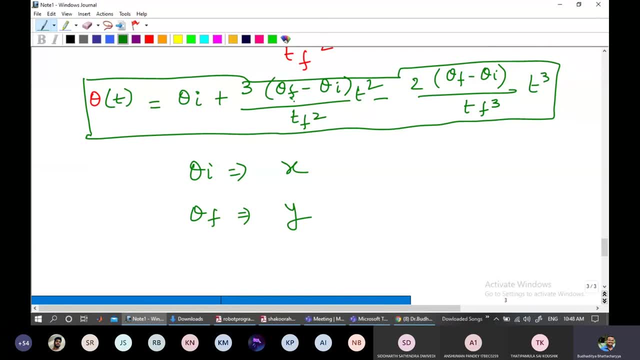 achieve is y. So if you can plug in these values of theta i and theta f and you give a time frame- t to t, t, 0 to t f- So we can find out what is the trajectory for the particular manipulator.